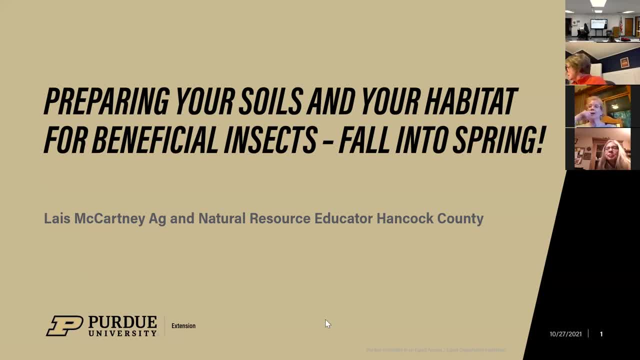 So, just like Mickey said, the fall is the perfect time to get ready for spring, actually. So, let's see, I need a support system. Can we help you? You want me to come up here and sit? Yeah, could you? That'd be nice. 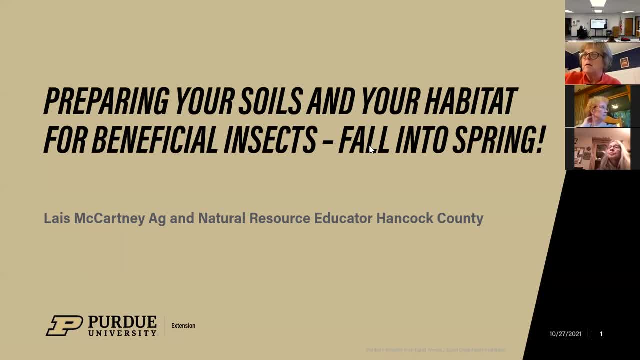 But the problem is my- oh, it's Peggy twice. I hope Peggy gets in now. The mouse: yeah, use this guy, Thank you, And then when you get done messing with the mouse, you can put it back over here. 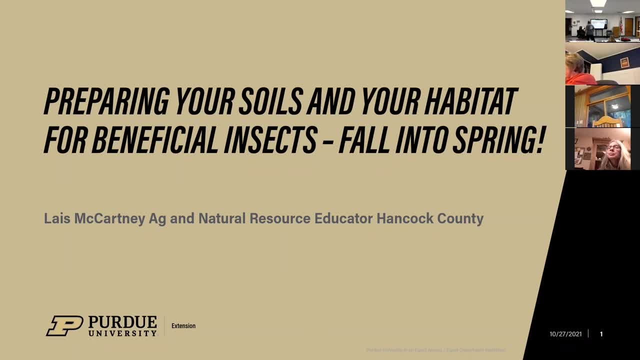 As long as there's no group on it, It might be, but I mean I try watching you. All right, let's see We need to do you just click this point again too. Can you use the mouse, Oh? 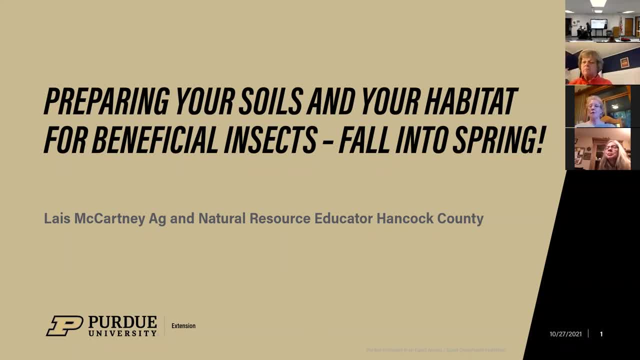 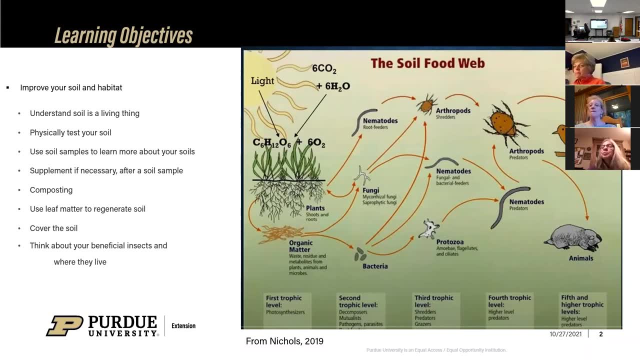 Oh, yes, Yeah, perfect. Thank you so much, Bob. Let me move this off here, Because this is going to be here, right here, on this side. I hope Peggy can make it in. Is she making it in? I just used the air. 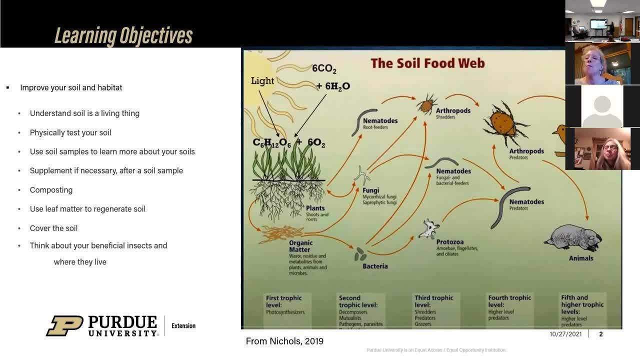 Okay, Basically, our learning objectives is: we want to make sure that we have a lot of time to do this. We want to improve our soil, which actually improves our habitat for animals. I know it sounds like it's two separate things. 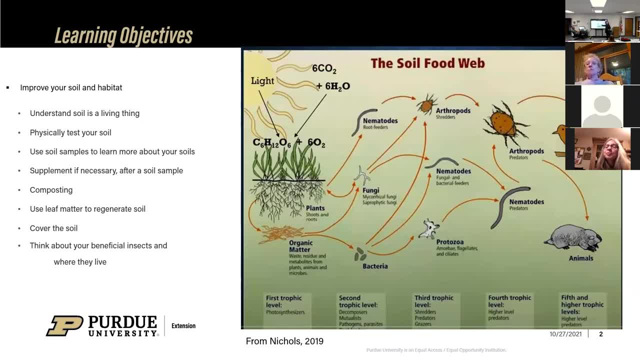 but our soil is actually where life occurs. That top soil, about four inches, is what keeps us alive every day. All the food comes from that, All the animals they eat from the garden and the yard and the pasture. They're getting all their nutrients from, actually, the top soil. 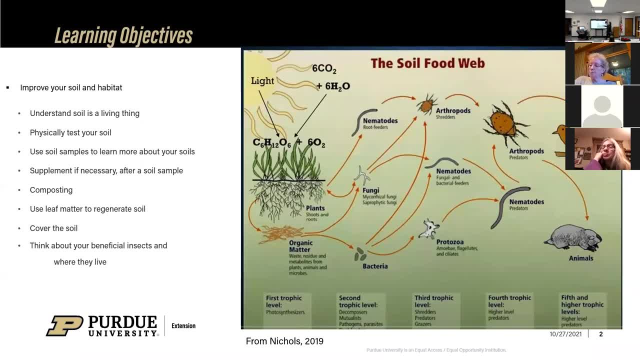 which is made up of a lot of different things, including organic matter, fungus, nematodes, all kinds of good guys. It's doing all of this to create living organisms. The soil is a living organism. We're going to talk about composting. 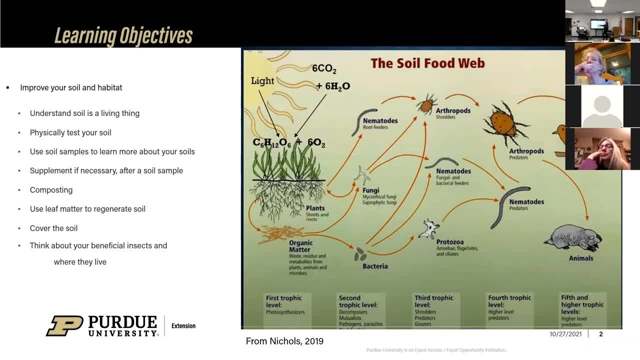 physically testing our soil, how to know what we even have. We're going to talk about supplementing, if necessary, only after you take a soil sample, because you can really mess up some things if you just supplement when we know. We're going to also talk about leaves. 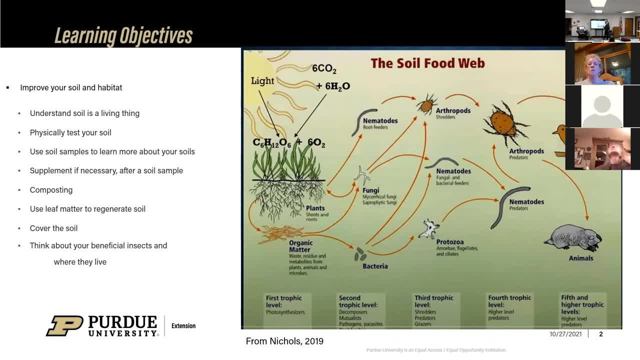 because this is my favorite thing to talk about- and leaves really are magical. They regenerate your soil. They're amazing. They are basically almost all carbon, and carbon feeds the microbes, which basically feeds the soil. It's amazing. So we're going to think about our beneficial insects and where they live. 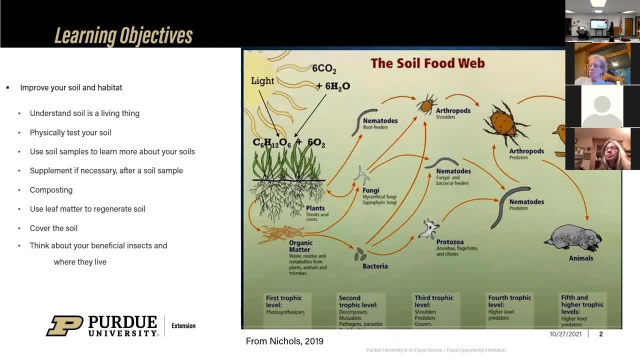 and they usually live in the leaves over the winter. Go ahead and use Bob's. Is that working for you? Of course not. So it's hard work, isn't it Bob? No, She's sweet, She's a great person. 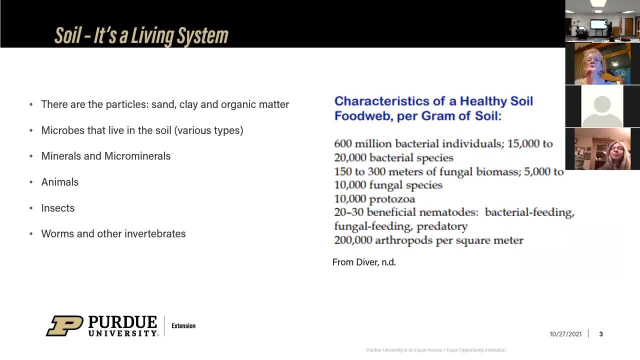 Yes, Just like I said, soil is a living system. In one gram of soil, which is really small, very small, 600 million bacteria are in there, Then 15,000 to 20,000 different species of those bacteria. 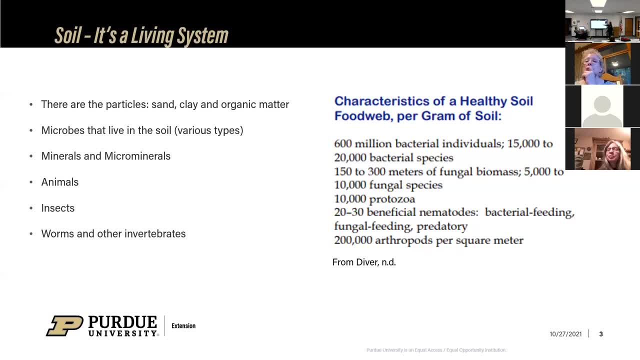 There's like 300 meters of fungus and protozoa and nematodes, beneficial nematodes. I was talking to Jerry about nematodes. He used to do research on nematodes And you know nematodes- beneficial nematodes- actually kill ticks. 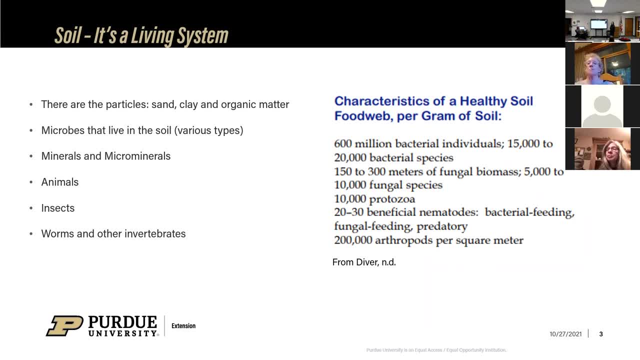 So the more beneficial nematodes you have in your soil, the less harmful things that will be around, because they're actually going towards those bad guys and that's what they eat. I think that's very interesting, So we don't need to be afraid of these things. 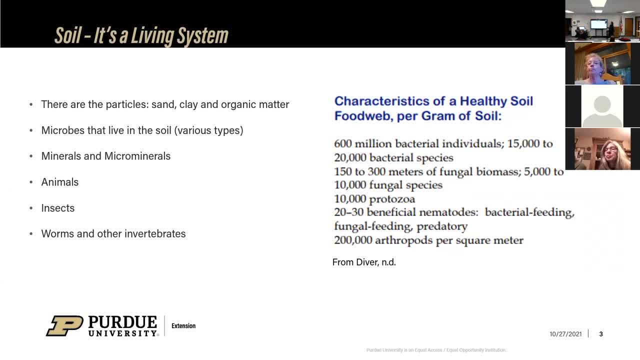 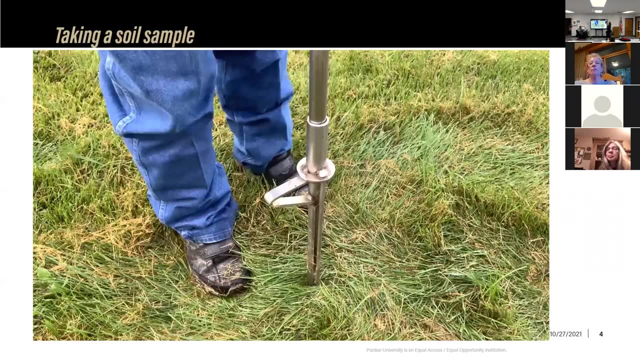 They're doing good things by eating some of our bad guys, So that's what they eat. Okay, So we're going to talk about taking a soil sample, because it's very important to know what you're dealing with in your soil before you do anything. 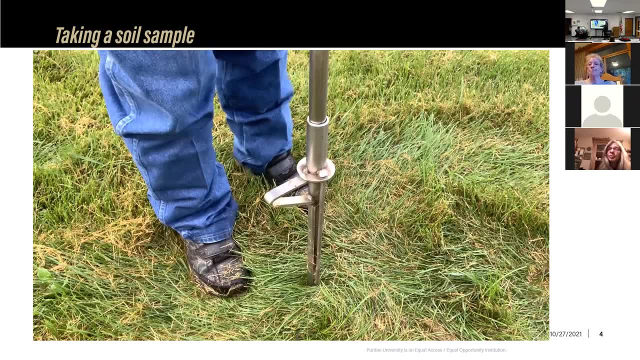 So this is a picture of a guy, Kurt Emanuel. He's using one of our probes. We actually have probes here. Has anyone ever borrowed our probe and done a soil sample here? Good, Has anyone ever tested their soil without using our probe? 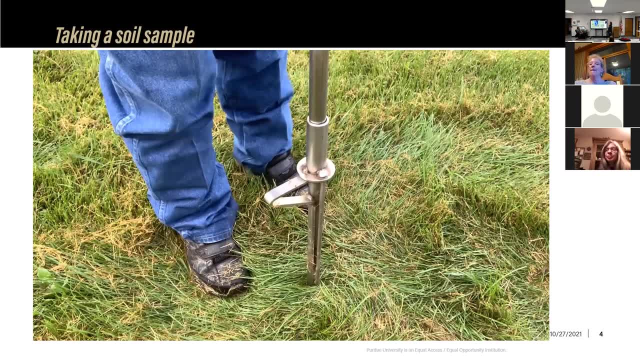 Awesome, Good. So there's just a few here that happened- not very many- And so this kind of basically helps to know what you're dealing with. A good time to do it is fall. You can do it right now And it costs about $20 to do the basics. 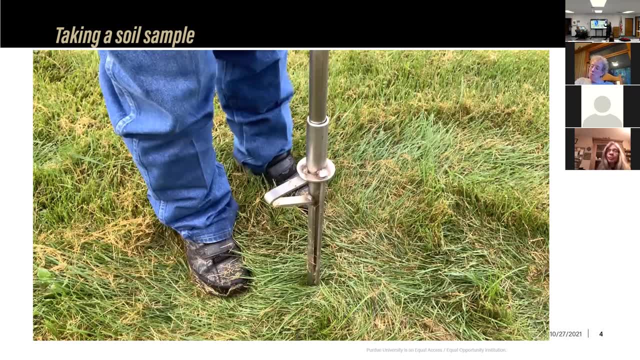 You can just get your stuff here to use and borrow And we send it to A&O Great Lakes. Well, you send it for $20, and you get back recommendations for whatever you're growing, For instance, if you're trying to grow a turf. 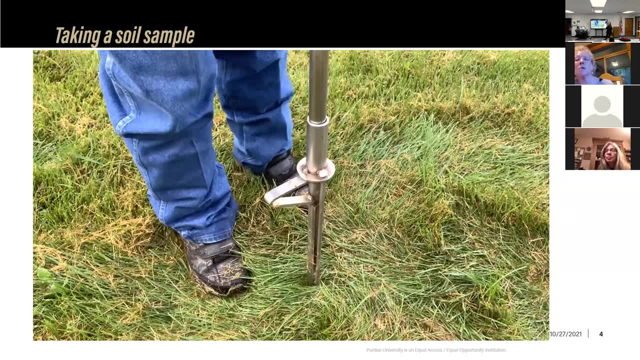 it might be different recommendations than if you're growing a tree. So talk to your doctor, Talk to me about it. I want to help you about that, But this is really important to do Basically, he just shows you how to do that. 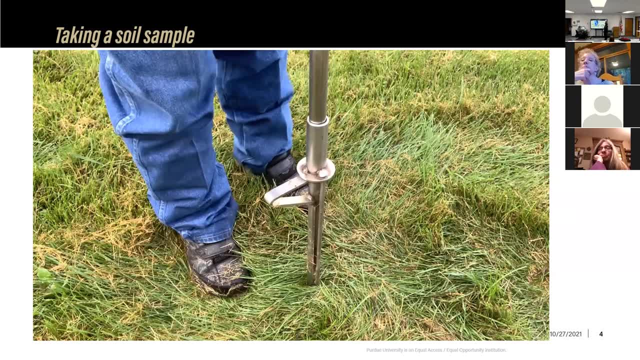 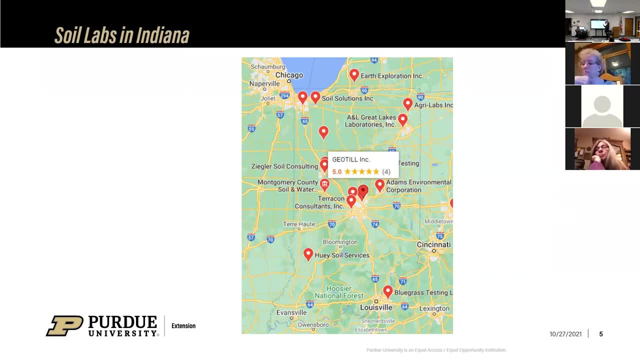 So let me know. if you have any questions about that, Go ahead. Oh, go ahead. Yeah, we don't need it. So there's different soil labs. You don't have to use the one we use And, in fact, there's different soil labs that do different things. 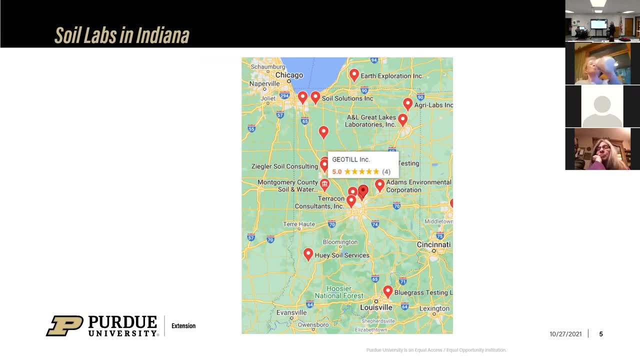 A lady called me the other day who wanted to know if she had been sprayed by herbicide, And she didn't know if her name had sprayed her tree And it died. But you can't just send that to any soil lab. You have to go to a place in Washington that does that kind of sampling. 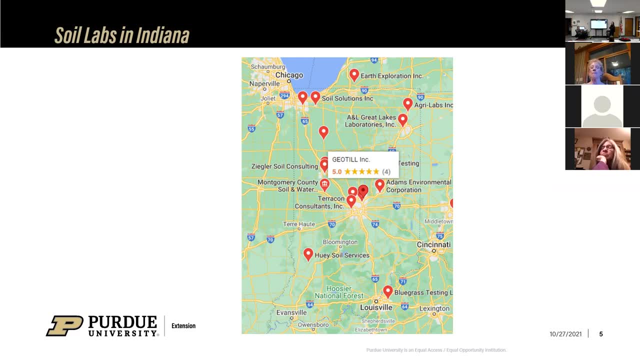 But it takes about. you have to check 500 different chemicals. That's a lot of chemicals And it costs a lot of money- about $400- to do this test, just to find out the vitamins on the side. So it depends on what you're testing for, what specialty. 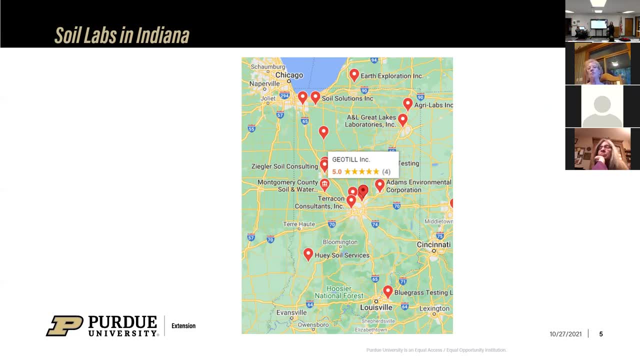 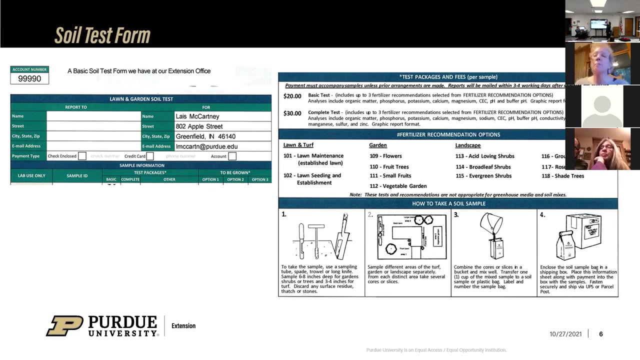 If you're doing compost. you know Great Lakes also does compost. Check that And test. so that's a different test than your soil test. So there's a lot of different options. Here's a basic soil test form. Just like I was saying, you want to say what you're using. 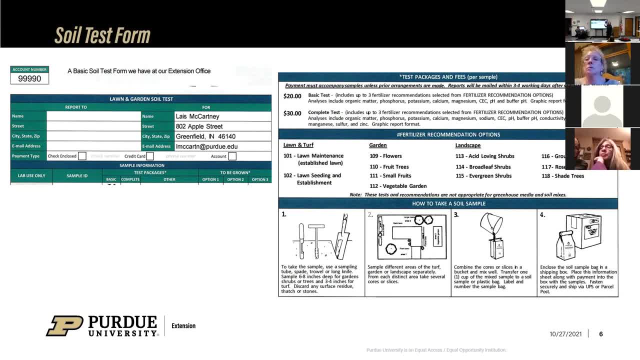 Wanted turf garden. you know landscaping, So whatever you're choosing, just say hey, I want to grow turf, And they'll give you ideas of what's going on. Go ahead. This is what's really important, No matter how much nutrients you have in your soil. 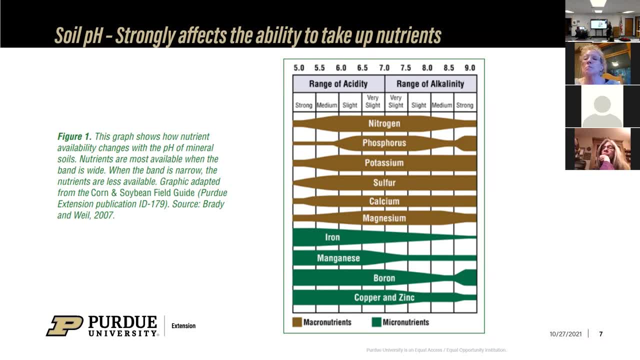 your pH is not in a proper place. Your plants actually cannot take up nutrients. They will starve to death, even though the soil is fertile. I decided it's a bad pH. So it just shows right here. I don't know if anybody knows what. does anybody know what pH is? 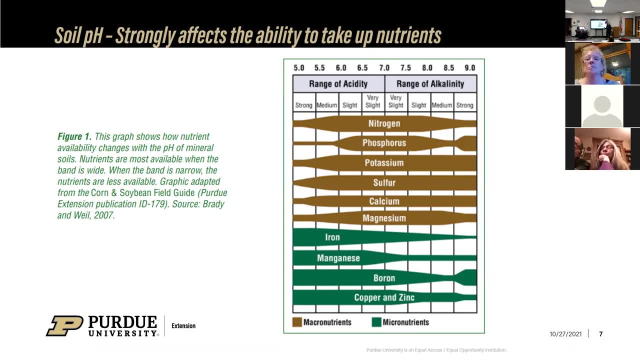 Awesome, Good. What is it? Can you give us a little gist, Don Do you mind? It's the alkalinity or the acidity of the soil, with 7 being neutral and 14 is on. I'm sorry, That's right. 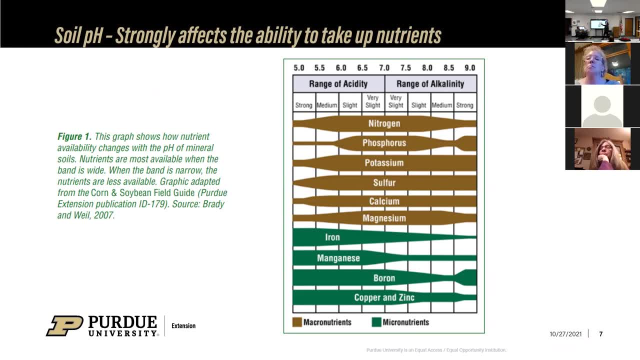 That's right. So 14 would be more basic, which would be over here, and more acidic would be over here. So this would be more like hydrochloric acid and up here would be sulfuric acid. So right in the middle, just like Don said, is the middle of it's called neutral or 7.0.. 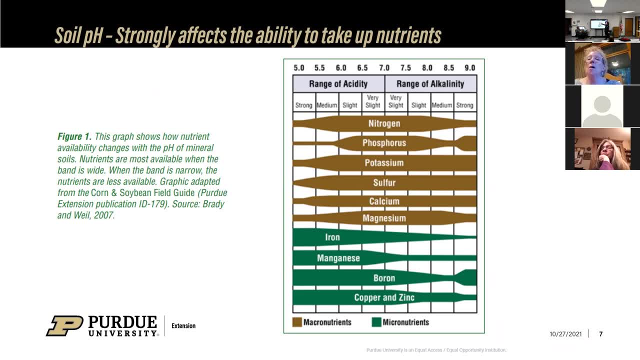 And basically right here can you see that this is showing the different types of nutrients: nitrogen, phosphorus, potassium, those big three in PK. Then you see calcium, magnesium. those are still some important nutrients. Then you're getting into the micronutrients. 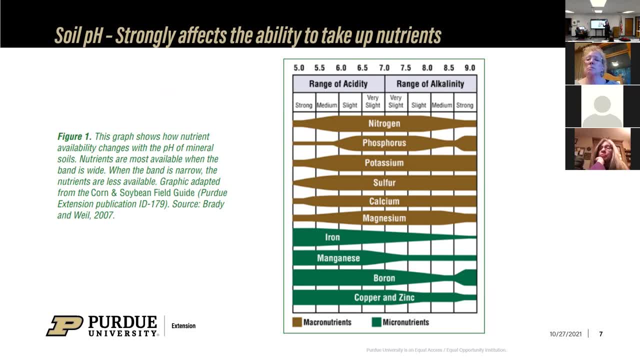 But do you notice you start getting high alkalinity, which is very, very common in Indiana soils. We're going to see some people who share their soil tests with me And you're going to see that we, because we live on limestone, that is a very basic material. 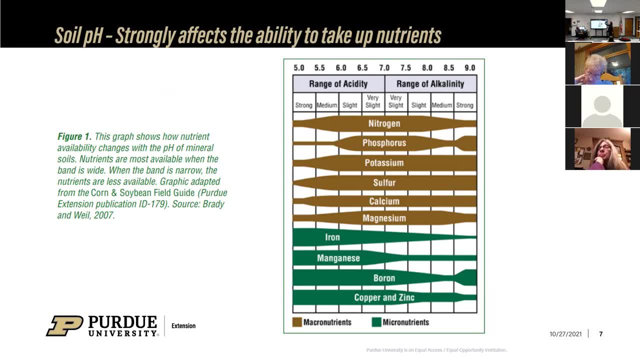 It's coming up to the ground and it makes us a little bit higher in our range of pH. So I'll see 7.5 pretty often. So if we were at 7.5, if you move down this, do you see what's happening with iron right here? 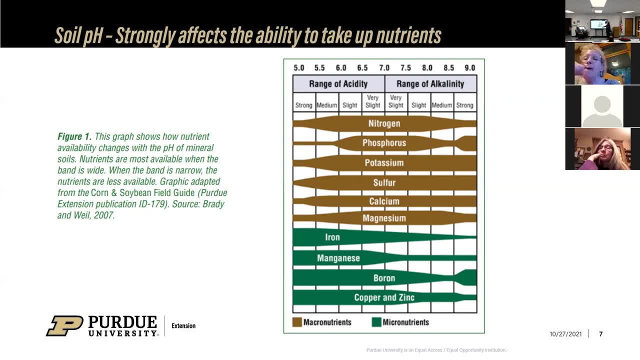 Do you see what's happening with manganese and boron and copper and zinc? So what happens? What is your symptom or sign if your iron is not getting uptake? Fruit won't set, leaves turn yellow. Leaves turn yellow, chlorosis, yes. 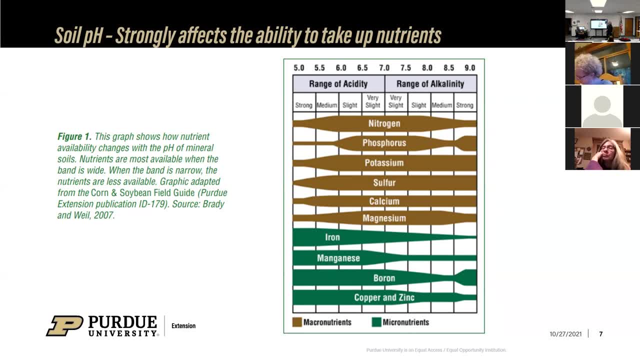 Has anyone seen that before? This is a very common symptom. This year, because of the excess amount of rain in my rain beds, I had to go and supplement with iron to get my fruit to set. Yep, Jerry said that he had to supplement because it was so rainy. it was washing out the iron or giving it. it was just basically overtaking some of those nutrients. yes, 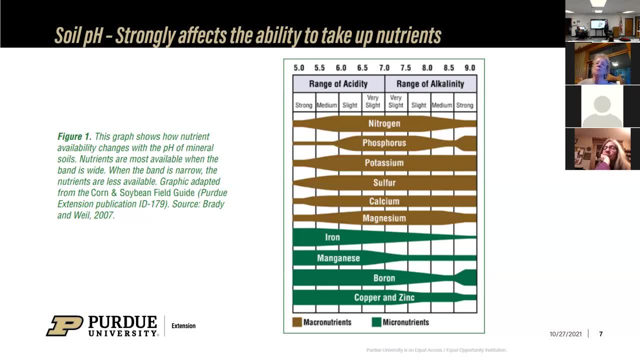 So that's why it's very important to stay within the proper pH and that's why you want to do a test. And you can buy those ones at Home Depot, but they're not very sensitive And they're also very expensive. But I would recommend that you buy them at Home Depot and you buy them at Home Depot. 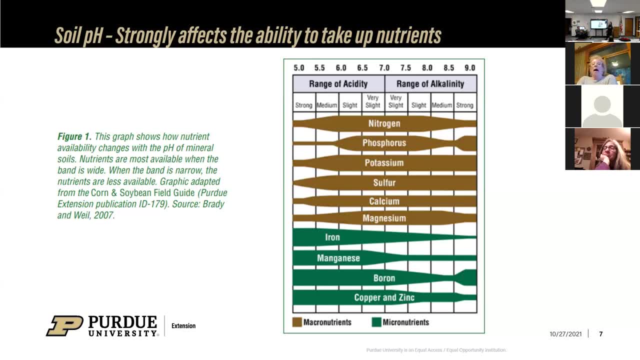 So there's not a lot of change, but there's still some improvement. So there's some improvements. I think the same thing I'm going to say is just the soil test. That's a little different than the soil test, but that's different. 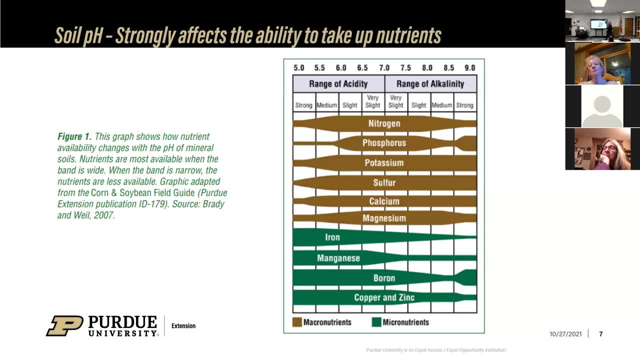 So the soil test is more accurate And, like I said, it's only $20 and they suggest doing a soil test about every three years to see how your soil is improving. And you want to do it around the same time of year because soil is similar at the same. 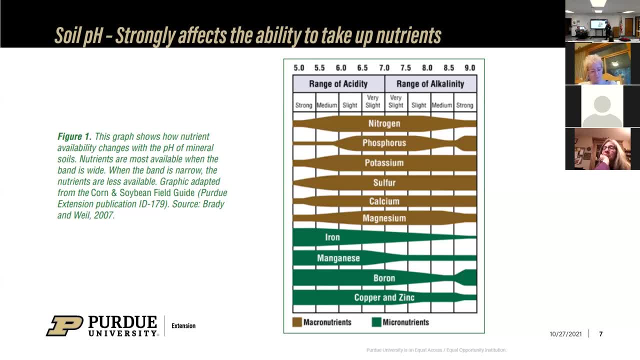 time of year. So here's a soil test result. It's a non-graphic, so it's not very pretty, but they basically have their sample ID, their lab number. That's just for the lab to keep track of, so they don't mix them up. 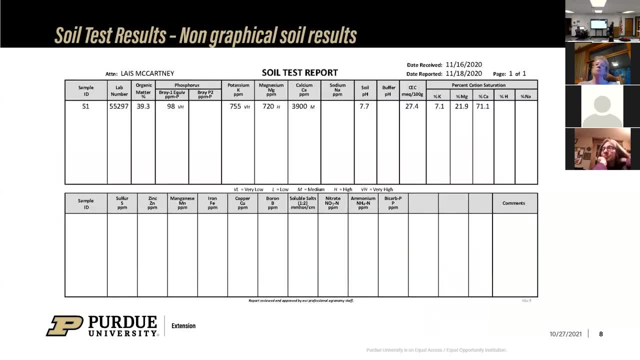 So here's a soil test result. It's a non-graphic, so it's not very pretty, but they basically have their sample ID, their lab number. That's just a lab to keep track of, so they don't mix them up. And they're looking at phosphorus: That's 98.. That's actually VH. 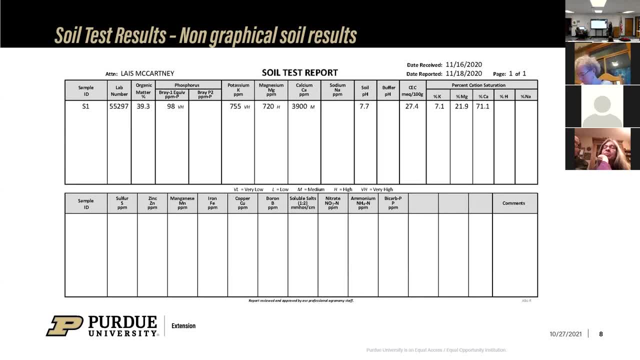 means very high. Phosphorus is easy to kind of get high, especially for using animal-based manures. Animal-based manures have a lot of phosphorus in them. So just because some is good, more doesn't mean it's better. So you have to remember that. That's why leaves are kind of 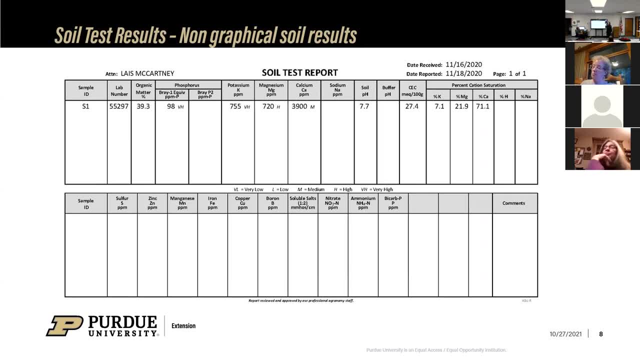 like amazing, because they do not have phosphorus- hardly at all. They have a very low amount of phosphorus, So you're getting that nutrient without overwhelming your soil with those phosphorus. It's not even as high as some things, but you just have to watch your phosphorus. 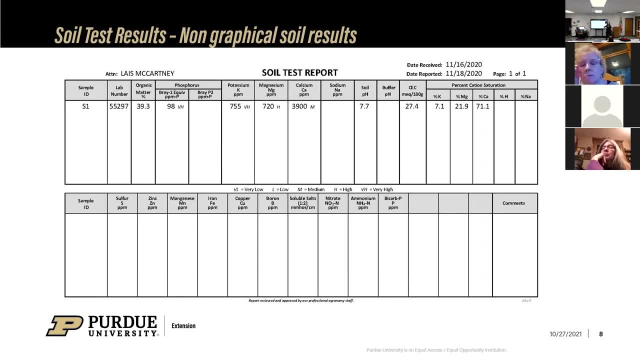 because phosphorus is what comes off into the waterways and causes algae blooms and causes epoxy in the Gulf of Mexico. That's why Fish are dying, because they, you know, lose their oxygen, And so we don't want to put too much. 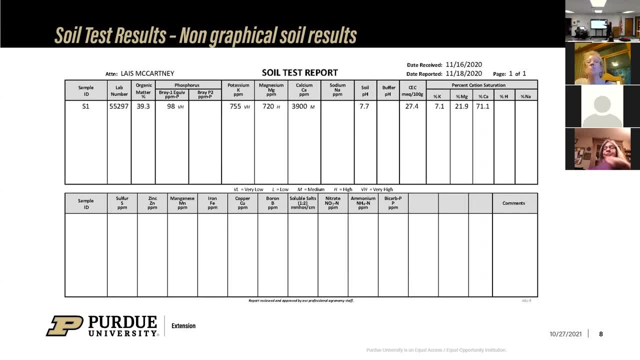 phosphorus to get into our waterways. Does that make sense? So here they're showing the potassium, magnesium, calcium and they're saying what? those are very high, high or medium. Here's soil: pH 7.7.. Where does that fall on the pH scale? Is that high? 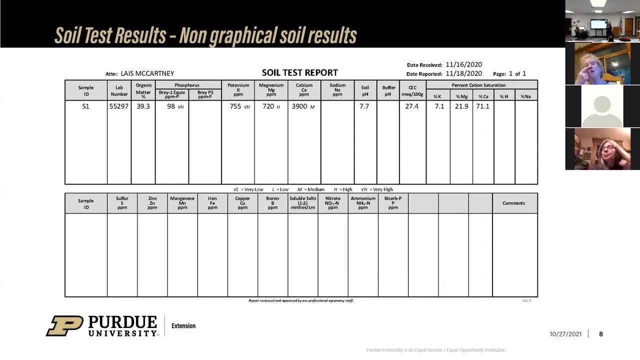 or low. It's alkaline. It's alkaline And that would cause what. Did you see how the iron looked? You wouldn't be able to uptake too much iron, would you? So this person is dealing with a problem with their soil pH, So they would get the suggestion to put. 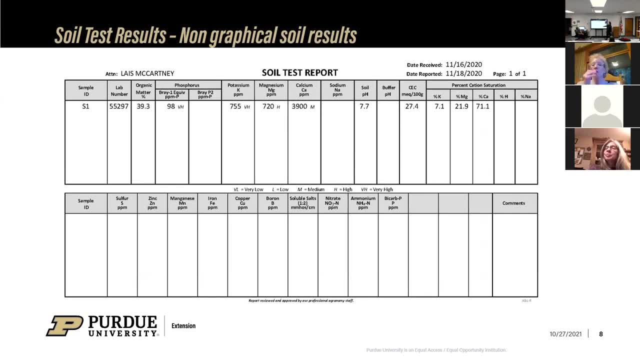 sulfur onto their garden and they would tell them exactly how much, but they don't say right here. But elemental sulfur will lower pH. but you can't do it all at once. You have to do it in increments over a couple of years because you could overwhelm your soil. So you just do it in increments. 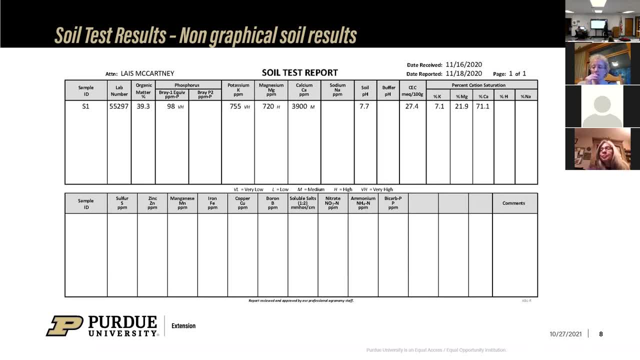 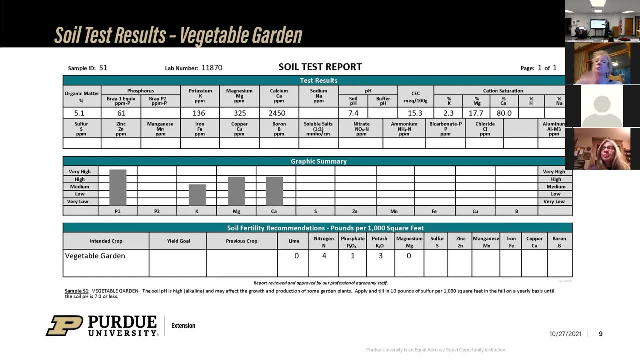 But they would tell you the amounts And how long to do it. Here's another soil test report. This person was wanting to ask about vegetable garden and their pH is 7.4, still high. Down here they say vegetable garden, the soil pH is high or alkaline And they want you to put 10 pounds of sulfur per thousand square feet in the fall on a yearly basis until that pH slowly goes down. They probably would want it to be around 7 percent. They want it to be right around the middle. That's where plants are most happy. 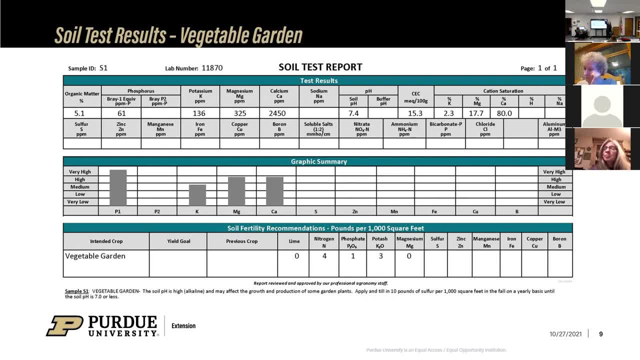 Now, how many people have always heard: put lime on your garden. put lime on your garden? Well, it's because the West Coast, they have more acidic soil, but they're also very big gardeners and they're like what's on PBS, And so we think, oh, we need to lime our gardens all the time. 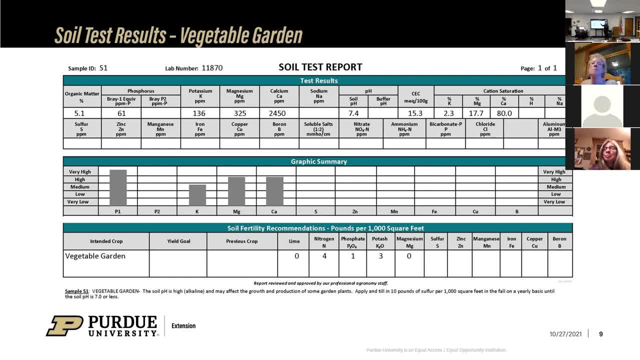 What would happen if this person put lime on their garden? Maybe their pH would go up, And do you know how long that would take? It would take about 10 minutes, And do you know how long it would take to get it back down? Very long, very long. 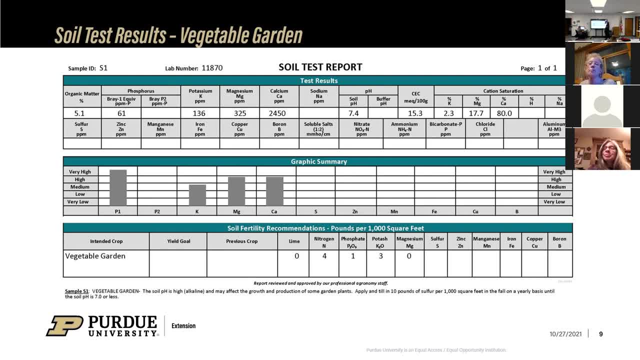 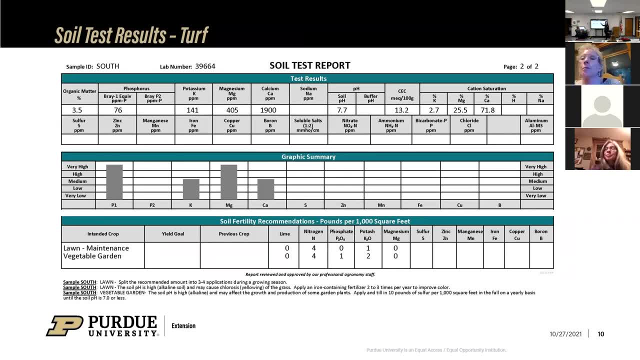 So be careful not to put things on your garden unless you need to, because it can take a long time 7.7.. These are all people in Hancock County, So you were dealing with high pH here normally. So never put lime on your garden unless you really really need to. 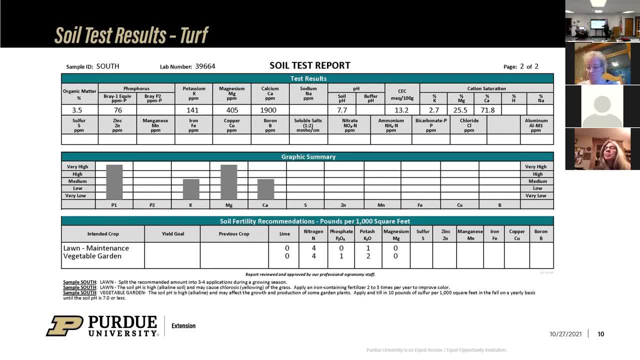 This lady came in the other day. She had horse pastures. She actually had acidic soil, which I really don't know how that happens, So hers was in the fives. Wow, I know. So guess what she did? do Put lime on her pasture. 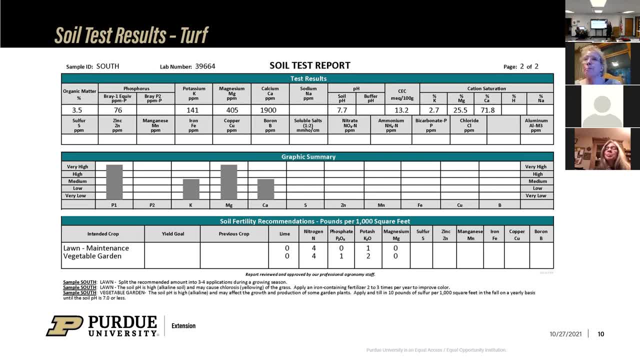 It's doing better, but it'll take a while to get that pH neutral. So that was. that was very unusual for around here. I don't know why it was, I'm not sure. I don't think she even put it on. I think she bought it like that. 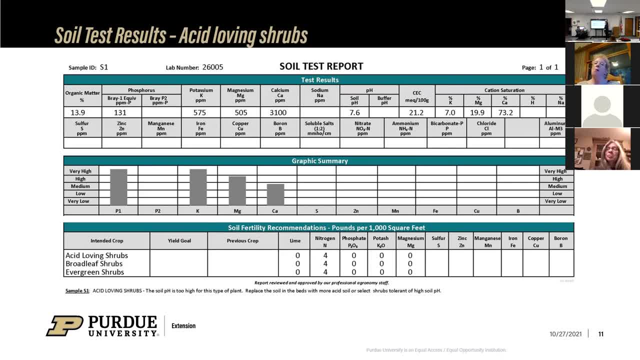 So I really don't know what it was on it for Go ahead. OK, here's acid loving shrubs. So an acid loving shrub Would we? can someone give me an example of an acid loving shrub? Hydrangea, sometimes depending. 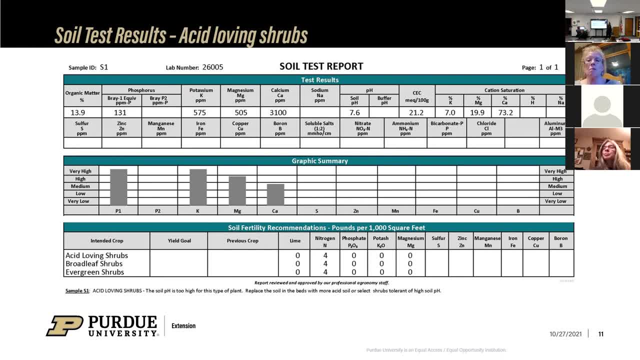 But what's another one? Everyone wants to grow these Blueberries. They always want to grow blueberries, And I hate to be the Debbie Downer, but they don't grow real well in our normal soil, So you have to amend or grow them in a container. 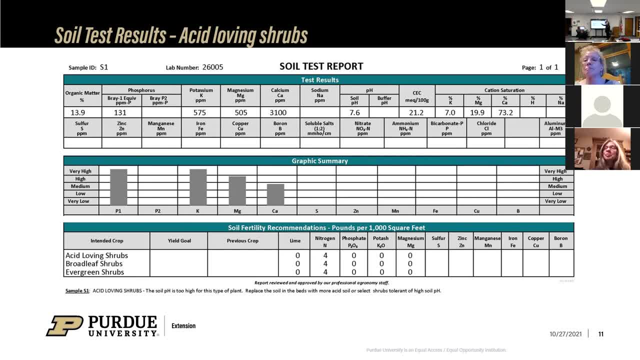 So this person has 7.6, but they want to grow acidic loving plants which are like around 6.5. So if that was going to happen, it says: replace the soil, The beds, get all the money in the world. 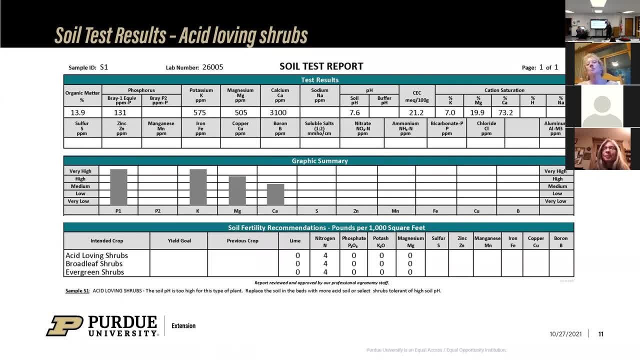 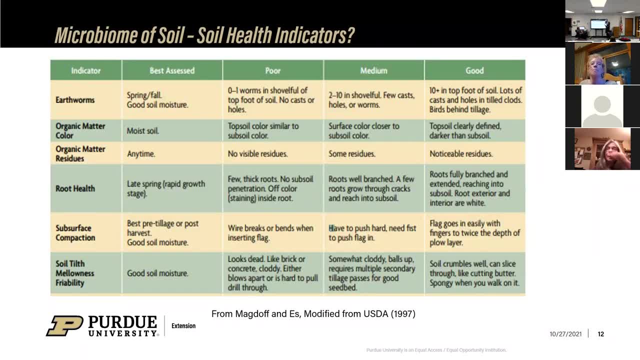 Or just know that we don't grow blueberries real great here, or community you know. so Here's some information about different ways we know we're having healthy soil. besides our soil test. First of all, just looking at your soil makes a difference. 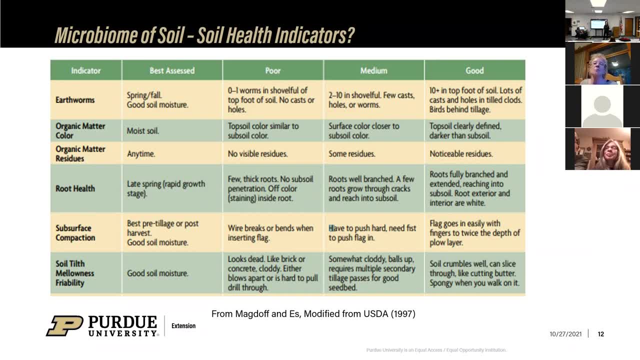 Do you have some earthworms in there? That's a really living soil. Now, if you're in wood, that's totally fine. Different ones usually don't have a lot of earthworms. Woods are more of a fungus based. 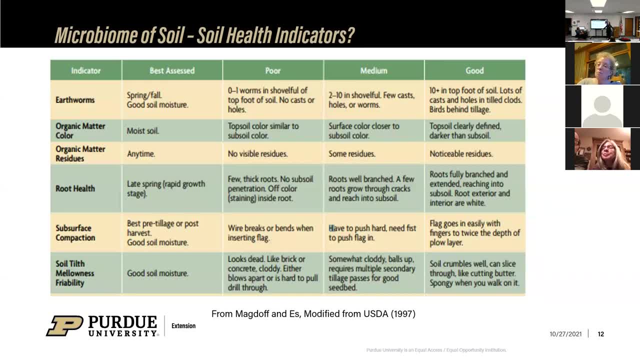 In fact they have networks and that's how trees communicate. They were the Internet before. it was cool, And they use their fungal networks to talk and to give information to each other. But worms are in bacterial soils, which is in prairies and normal turf. 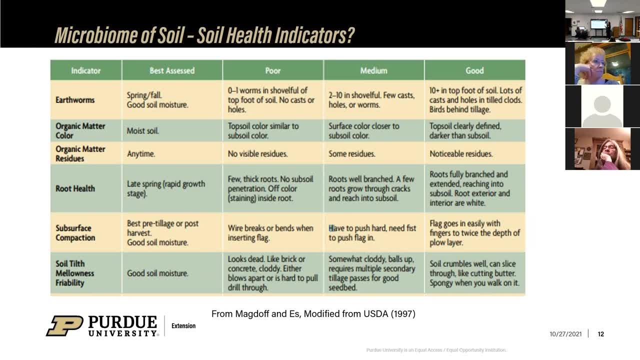 And what we usually deal with. we're not usually dealing with woodlands, But if you see earthworms in your soil- about 10 in the top foot of soil when you first get like a shovel full man, you're doing great. 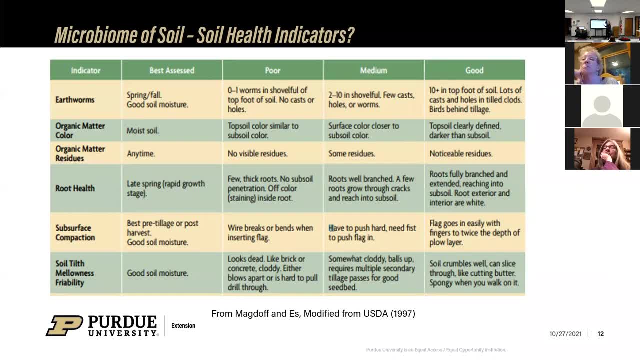 So that's a good way to know. Also, your tops Go ahead. Does someone have a question? OK, Top soil is clearly defined. It's darker than your subsoil. That's good. Now, remember this might take a while to get to this point because, let's be honest, when we buy our homes in suburban areas, 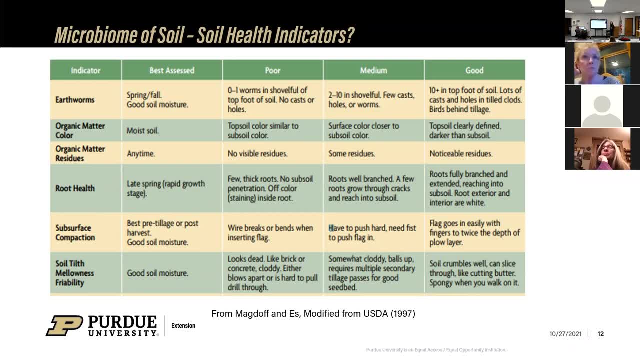 what they've done is they've actually stripped the topsoil, sold it to make some money. They probably kept some of it, but they didn't keep probably all of it. They're supposed to keep the soil stocked How we? you know we check that in our planning. commission notes. 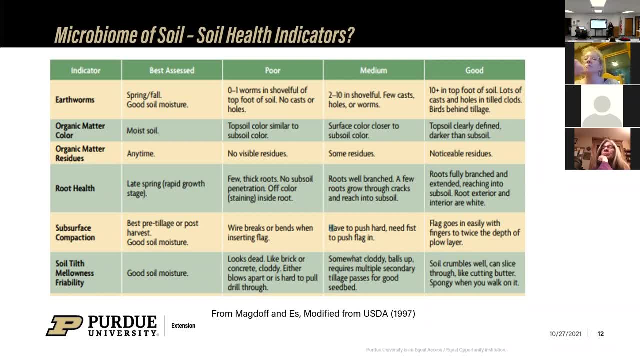 But you know, and it just there's sometimes just a little bit and not much. but you're dealing with a lot of just not topsoil, So you have to build that back up and it takes a long time. Some information about organic matter: If you see some residues, that's a good way to know that you have some. 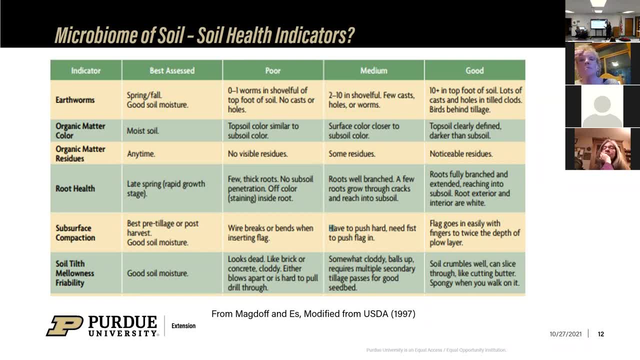 Living soil. but that's hard to do sometimes because if your microbes are hungry they'll eat it all. So it just depends. Looking at your roots of your plants will teach you, tell you, how good your soil is. Have you guys ever pulled out your plants and it's like, oh, they're so big, that's a really healthy soil. 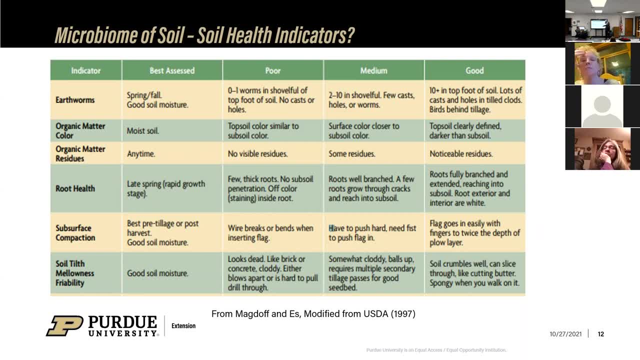 That's a good sign. If you can start putting your hand in your soil without hitting anything, you start looking like the man from the PBS station, like Liberty Garden or whatever that guy who was like. he put his hand all the way up to his elbows. That's totally a great soil, but that's hard to do. 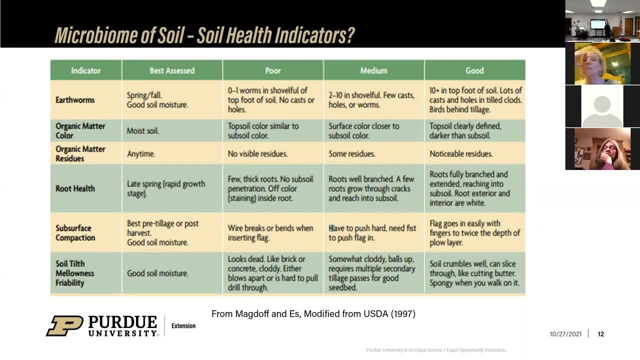 And then when you hold your soil, what's it like? What's the structure like? You want soil that holds its structure and it crumbles a little bit And because that is meaning that has aggregates, it can hold water and it's holding those nutrients in there. 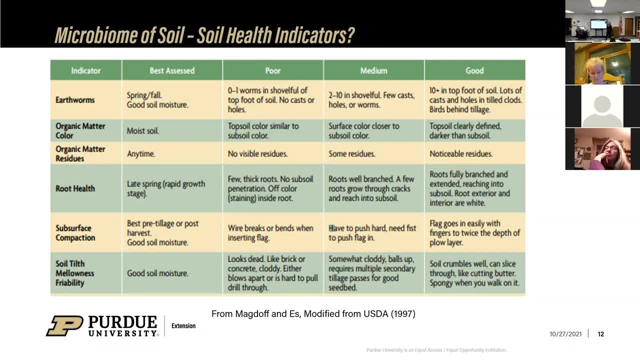 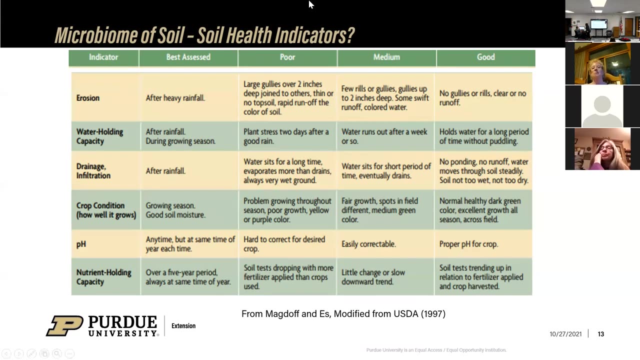 So we have really good soil around here. even though it's clay, it holds a lot of good nutrients, if it's healthy soil. I'm going to check some things before entering the waiting room. Let's see if it's three pegs. 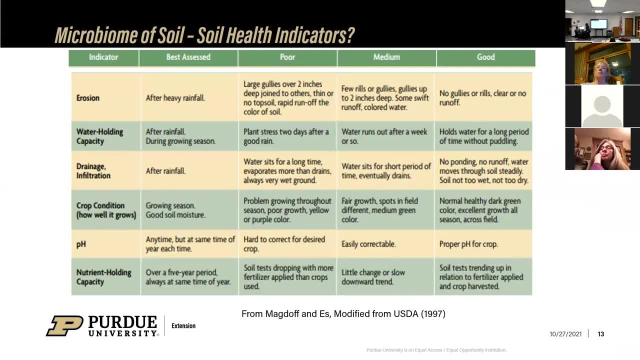 Yep, it's two pegs and Susan. let's see if it works. Here's some other soil information. Are you having erosion? If you're having erosion, that means your soil isn't holding itself together very well. It's like falling apart. 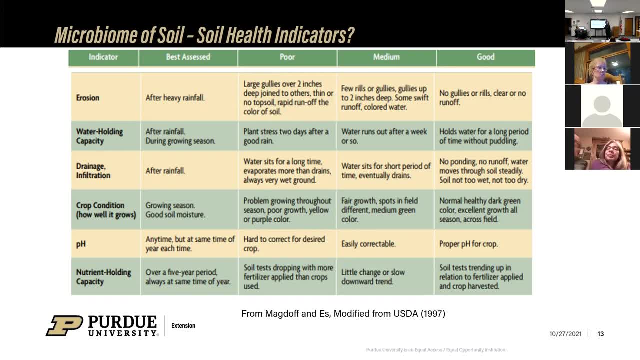 So if you're getting gullies and stuff, that means your soil is unhealthy. But if you are, you want to look after rainfall And basically, if you're having very few gullies, then you're better, But if you get a lot, that's bad. 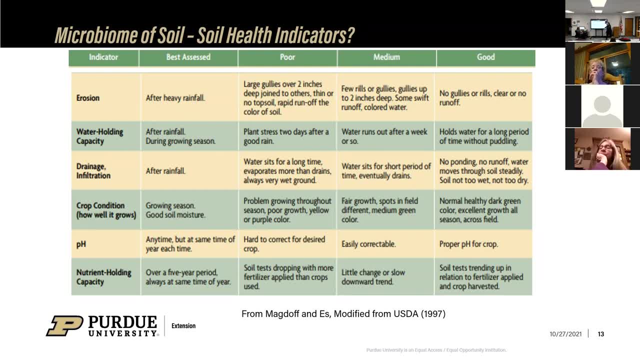 So no gullies clear or no runoff. So basically, when it's running off into your ditch, is it clear or is it bringing dirt with it? Because if it's bringing dirt with it, you have unhealthy soil that's not keeping itself together. 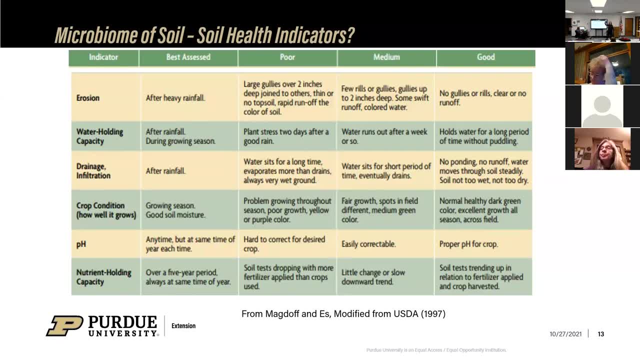 Water holding capacity. this is so amazing. So did you see the rain garden out there? We've just planted it. It has not been in there for even a month yet. It just got planted at the end of September. Those plants, even though they're not grown up, they will hold 30% more water than the turf that was there before. 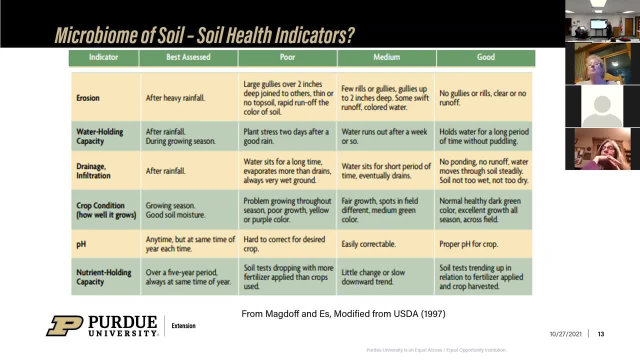 So I don't know if you guys ever saw when it would rain. there would be a lot of water right there. It would take forever to go in. So plants and healthy soil hold more water And we'll just make sure. nutrient holding capacity obviously increases when you have healthier soil. 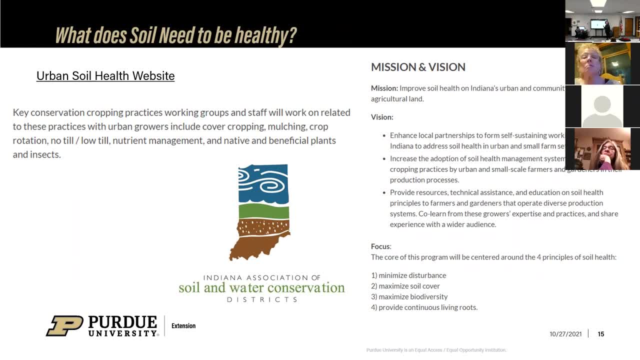 So this is really neat: The Urban Soil Conservation, which is part of the Soil Water Conservation District. they're all about helping backyard gardeners with their soil, Because they realize that there's a gap. Yes, NRCS and Soil Water Conservation: they're helping farmers with their soil. 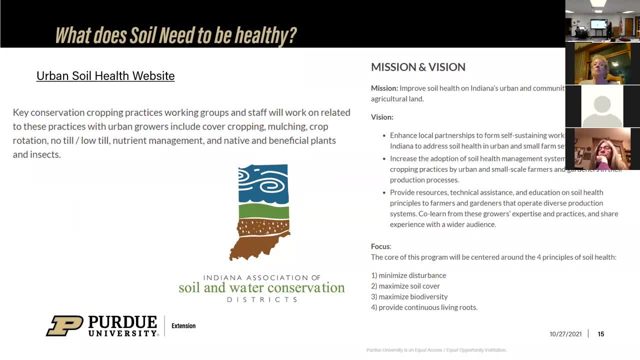 But we also need help with our soil And we need resources. So actually they have a mission and a vision. They just started a new statewide program for the Urban Soil Health Association with the Soil Water Conservation District And their whole purpose is to minimize disturbance. 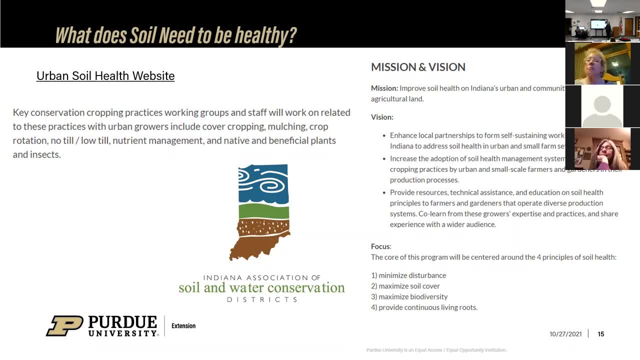 That's how you have healthy soil, Just like- remember Teresa was talking about her tilling of her pollinators- Her pollinator garden Tilling actually brought up a lot of weeds, But it also hurts the soil structure. Then maximize soil cover. 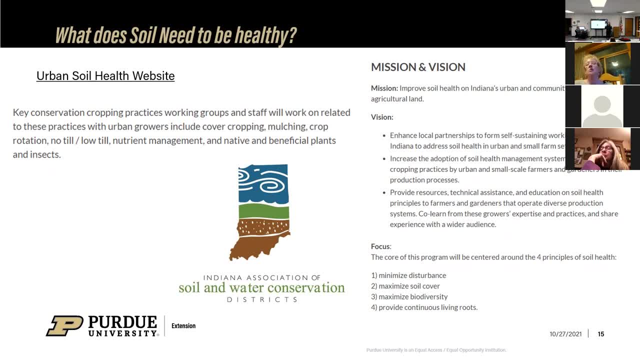 Because if you keep the soil covered, you're first of all helping plants to be covered for the winter, And animals and insects, But you're helping the soil because the soil is alive. also, It kind of gives them a blanket over the winter. 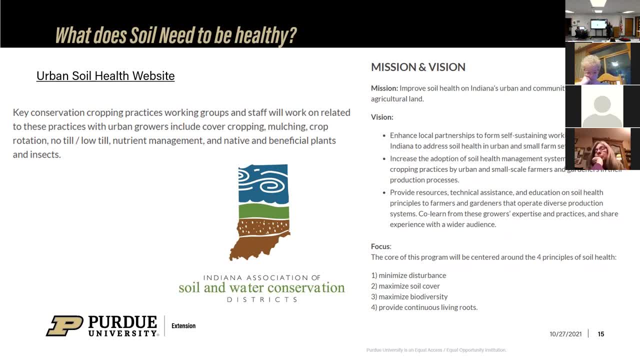 And it's good to keep soil covered over the winter Regular time of the year, Why do you think the summer would be good to have your soil covered? What do you think happens in the summer? They dry out, They dry out, Yep. 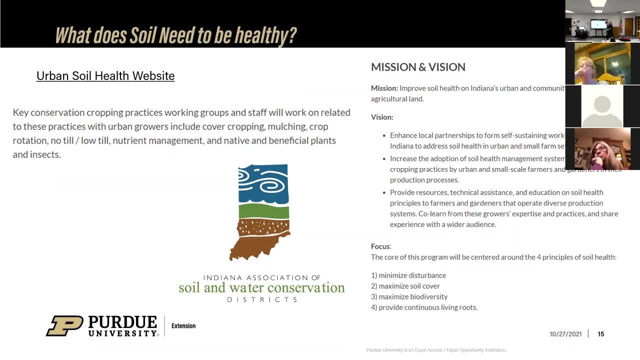 It has a lot of transpiration. It gets all that water out of the soil. But if you have like a little blanket over it, you're protecting the soil from losing its moisture as easily. Maximize biodiversity, Which basically is maximizing the microbes in the soil. 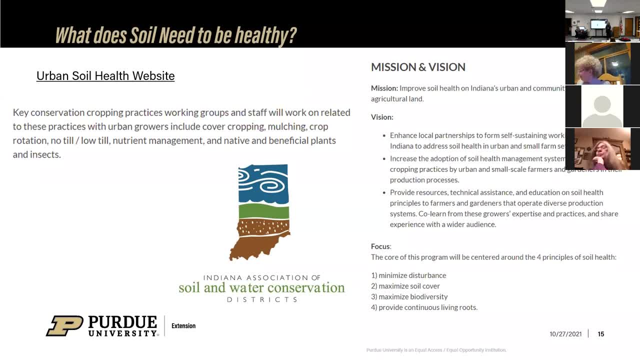 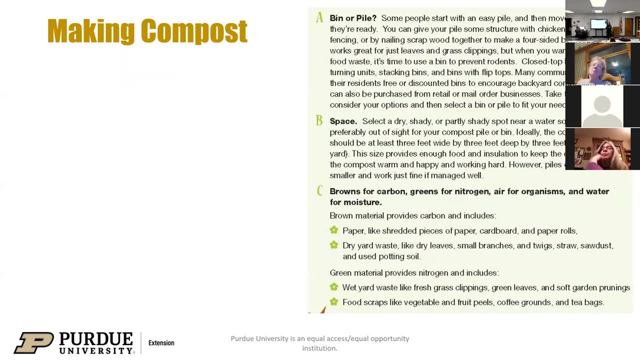 And provide continuous looking roots, Because it keeps the soil together better And you have roots always in your soil. Okay, That's why you're noticing a lot more farmers. They're doing cover crops And they're starting to realize they don't want to lose their soil either. 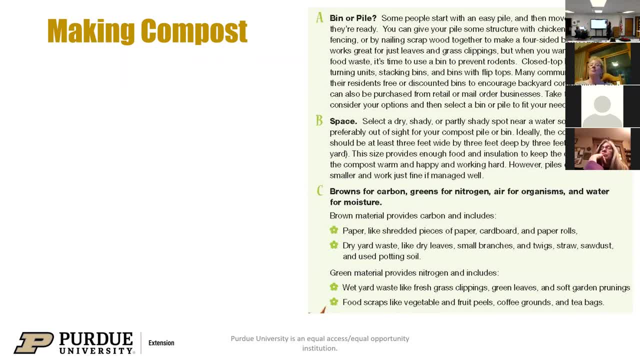 And they don't want to see it going down the creeks. But it's also scary because it's a whole new way of thinking, So it's going to take a little bit. So let's talk about compost. Compost is a way to cover your soil. 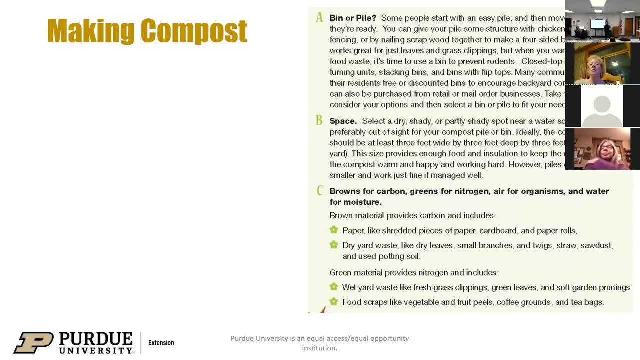 What is compost? Does anybody compost here? Marianne does, Yep, Okay, cool. So, Marianne, I know you do leaf compost, Which I have a video of you on here. Do you do any other green compost with your? We have a major composting at my house. 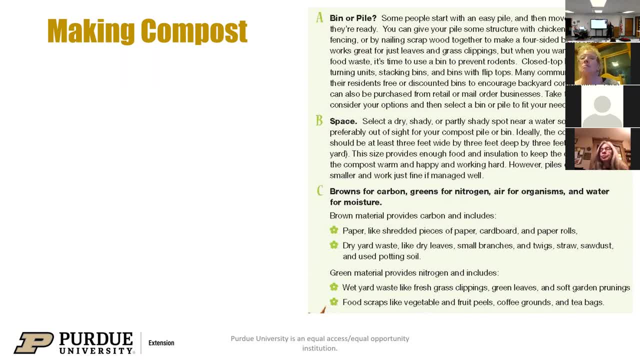 Lots of leaves, Lots of leaves, And then we put grass clippings in it for the green, And then we put any kind of scraps from the kitchen that are not in the leaves. Good, Awesome, Who else Don do? you also do it. 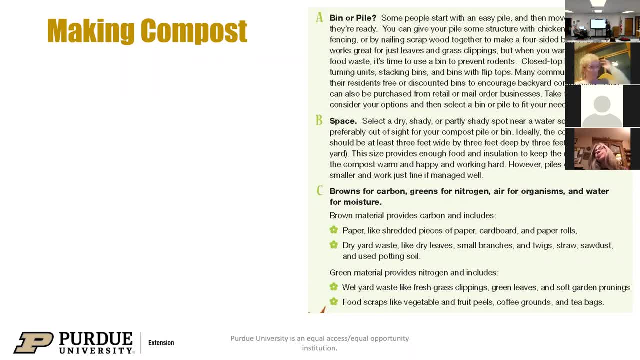 Pretty much the same thing. I do have a question, though I don't turn mine because it's too much work. You're after my own heart. I'm the same way. You do not have to do that. If you want to work really hard and have your compost faster, you can. 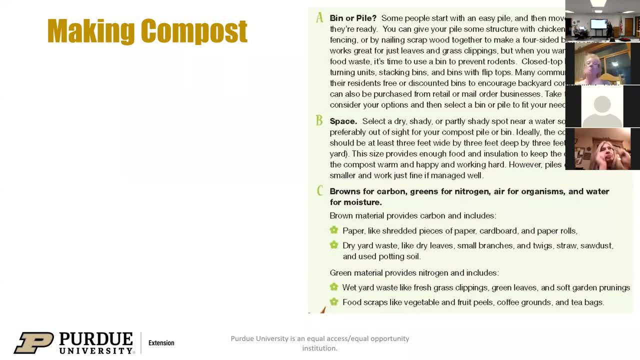 But you really don't have to. It just takes longer. It takes about nine minutes or a year to cook down. Yes, But you know, the fastest way you can do compost is if you have about a yard cube and you turn it every day. you can get it done in 18 days. 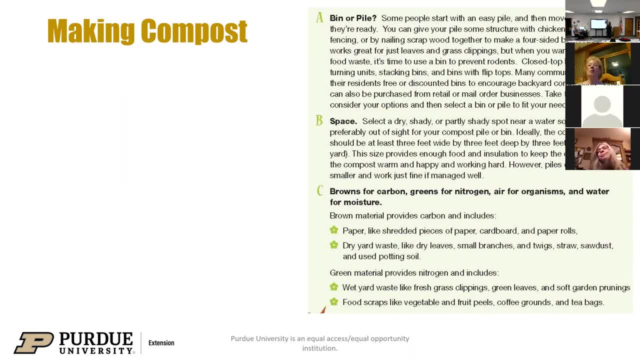 Okay, And when I say done, done, you just know it's done. First of all, it got into a heat. that was correct. There's a temperature, We actually have a compost. I don't know if you want to borrow it, because it kills pathogens and stuff. 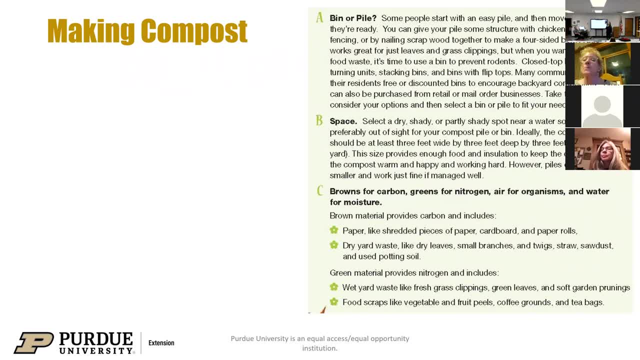 But then you can do it if you really want to work really hard, But I don't like to work very hard. Yes, Marianne, I have a question, Yes, About compost. So we compost majorly, And I even have some left over. 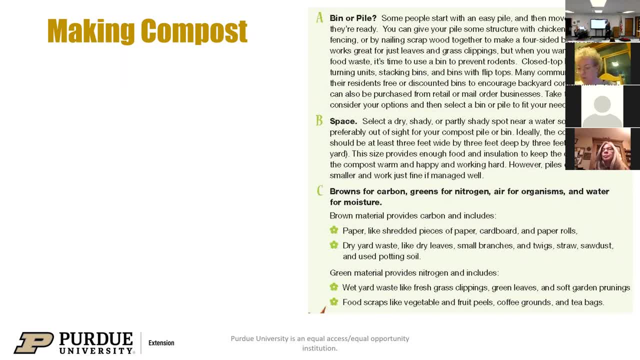 I took it on the pantry, which is like really cool. Yeah, So the plants that we planted- I provided some compost on top of that. Good Good, I have so much that we're kind of using like stuff from. that was from two years ago. 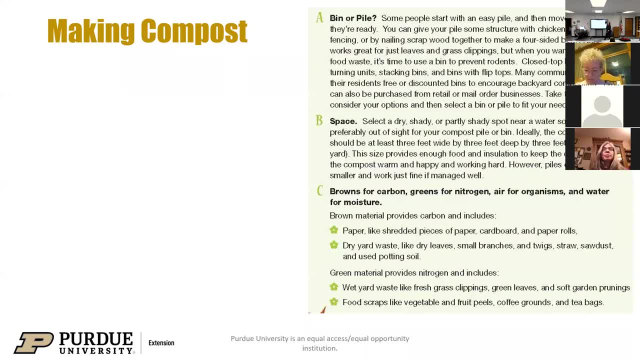 So is it okay if it just sits there? Yes, Totally. For some reason, I got the information and something leaches out of it and it's not as good anymore. You will lose. So here's the thing: Potassium can leach out. 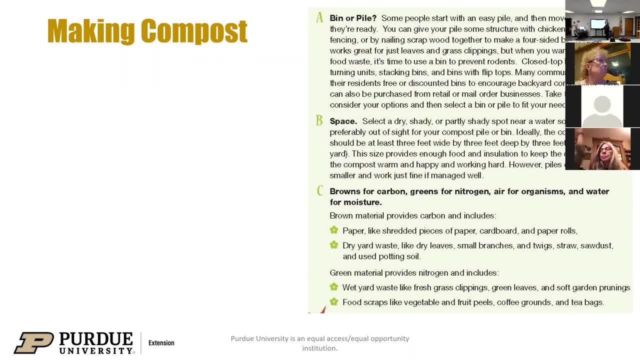 Yes, Potassium can. So if you really needed potassium in your yard, Some people actually put a tarp under it so they don't lose it. I know it sounds crazy, but potassium moves fast. Phosphorus does not move fast in soil. 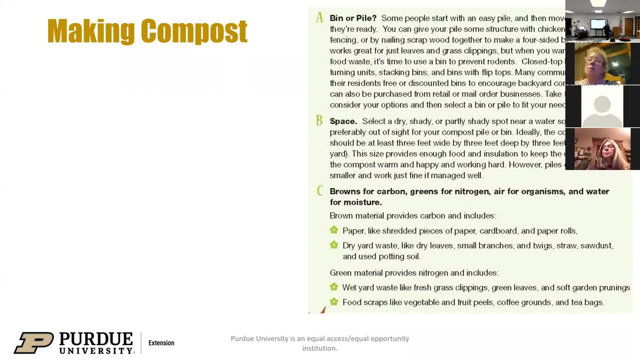 Potassium will just kind of drain out. But you know you can only do what you can do. Don't feel, Don't be afraid of it. There's usually enough potassium in our soil to be okay. But if you were dealing with, like in a sandy soil that you really needed to preserve that potassium, you might put a tarp underneath your compost pile. 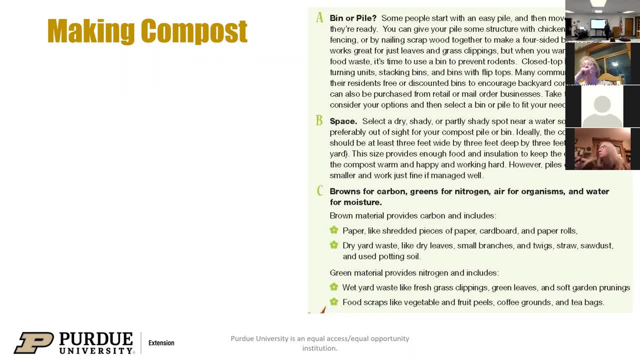 And then you would not lose your potassium. Does that make sense? So it kind of depends on what soil you're dealing with. Yes, I have a question. I thought I heard somewhere and I've been doing it, And like garden fertilizer, like 10-10-10, your compost, that helps speed up the process. 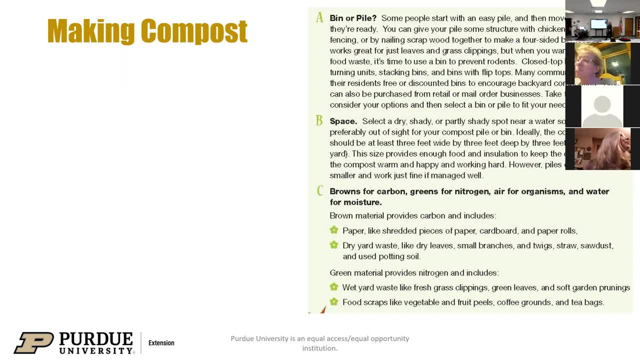 Or if you don't have any of the grooms, all leaves, I'd be careful. just because of phosphorus, I would test your soil, Do a soil sample, Because if you do tests, Because if you do 10-10-10, that's nitrogen, potassium and phosphorus. 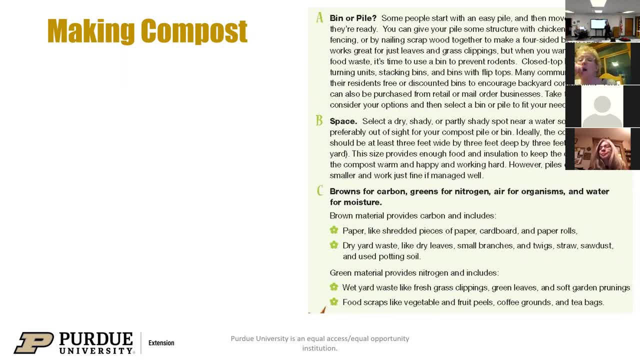 If you burn nitrogen, phosphorus, potassium- whatever you want to say- and PK that phosphorus, you can get too much, And getting too much is it can cause other problems. It has to be pretty high, But if you're just doing that over and over again, it can add up. 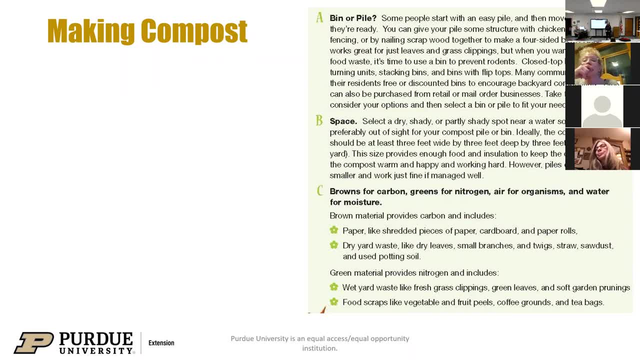 And you might not need that much phosphorus. Does that make sense, Bruce? Yeah, If you just go to the co-op, buy a bag of straight urea Which is nitrogen, Yeah, That might be better And you just take like a cup or something. 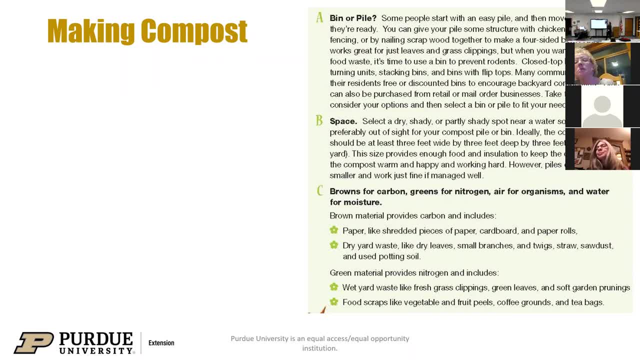 If you've got a small compost pile, Just sprinkle a little bit on there, Mix that in a little bit And that pile will heat up pretty quick. Yeah, Yes, And that might be better than around here We may have too much phosphorus. 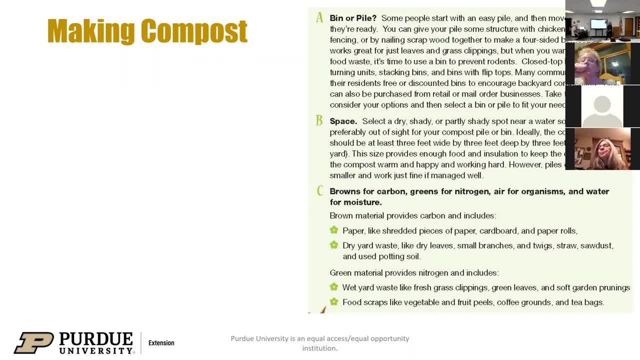 But it depends on where your soil is. So that's why it's good to test it before you just add things. Then you're just getting straight nitrogen. Yeah, Nitrogen, That only helps it. Yeah, Yes, But you are right. 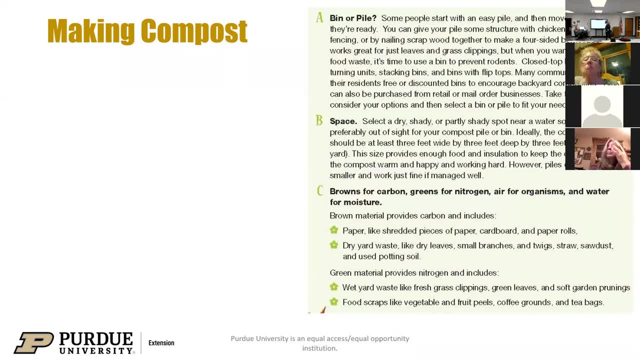 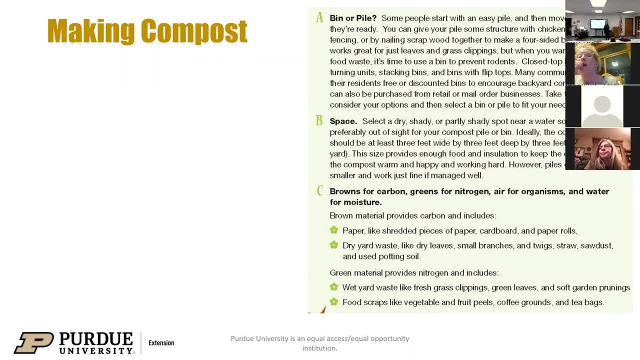 And you're using the microbes to break it down, not necessarily the chemicals. So, just like you probably know, when you have hay you don't want to put it away wet because it can start a fire. You know plants have energy and they can start things burning. 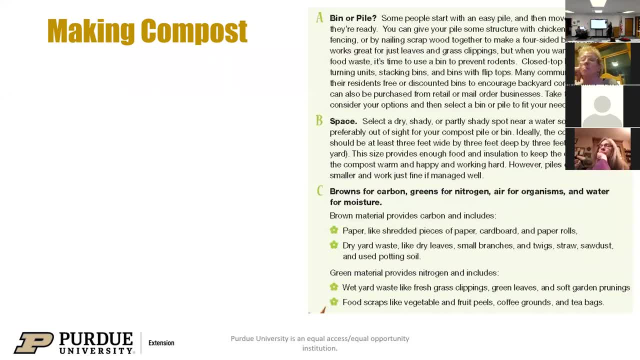 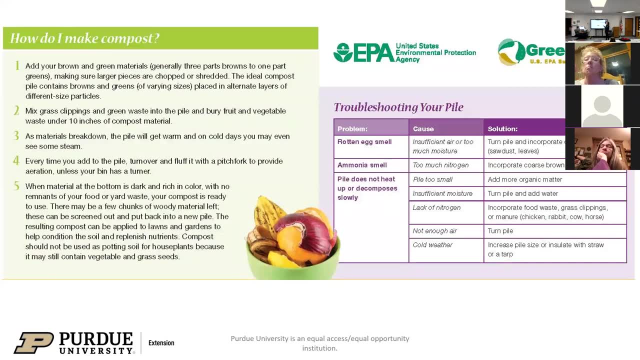 You know what I mean. It's amazing. Yes, sir, Yes, it is. So, basically, EPA tells us how to make compost. They want us to make compost because we waste, first of all in the United States, a lot of food waste, and it just 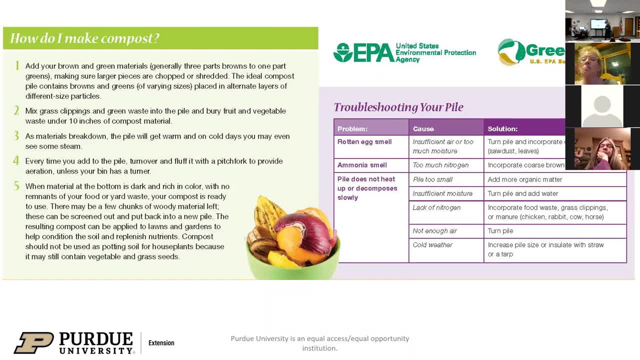 goes to landfill, whereas the nutrients could be used to help our gardens. So basically it just talks about you want your browns, which are like your leaves, or the carbon. You want your grains. just like Bruce was saying, sometimes you don't have enough grains If you use some yard waste. 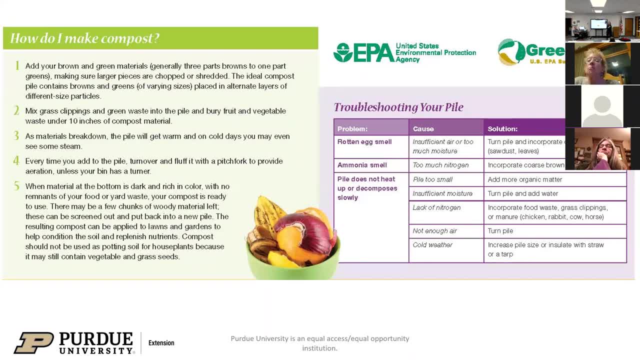 like any green leaves or your green grass clippings. you could do that The only thing with green grass clipping. time people have done a whole big pile of green grass clippings. and how did it smell? It stinks up to high heaven and your neighbors are like: why do you do this to me? 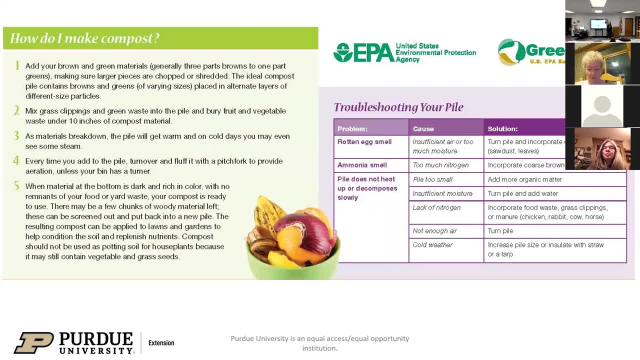 So don't do that to your neighbors, but it does work. It does work and it will be a lot of nitrogen. So that's just an idea to get some grain stuff in there. Go ahead And it's okay, I'm sorry. Question. 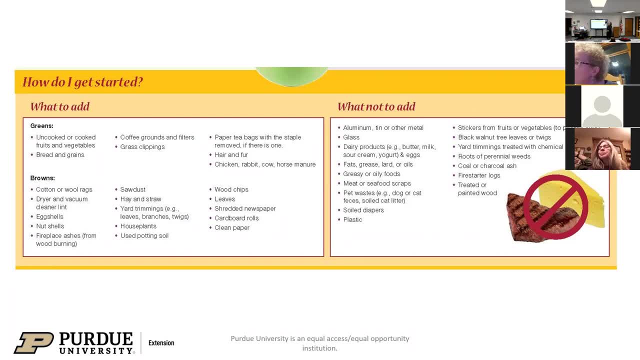 It's okay to put seeds of things. like we've been cutting down the honeysuckle. I've not been recycling it or composting it. I've been burning it because I don't want seeds to and we don't have very active compost, So it's okay to put the seeds of plants in there. 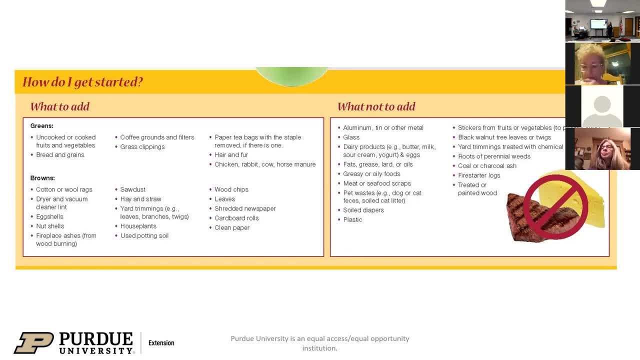 That's a good question. People get iffy about especially invasive plants because it depends. You can always say it depends and that your compost can't have enough to kill the seeds. You know what I mean, And so it's hard to say. They probably just say no overall, just to protect you. 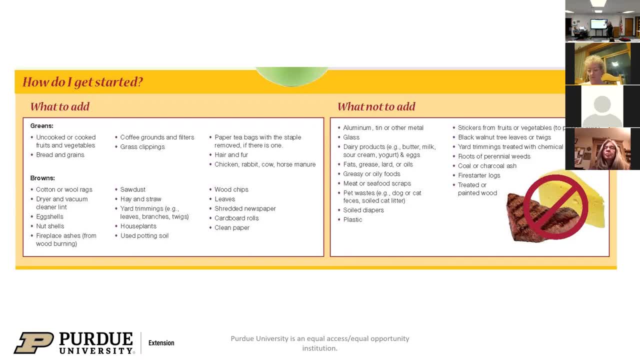 because they don't know how hot your compost gets, or even how you do your compost, or if you're adding green to make it hot, And I did that close to 160.. It's not going to kill the seeds. Okay, correct, Yes, 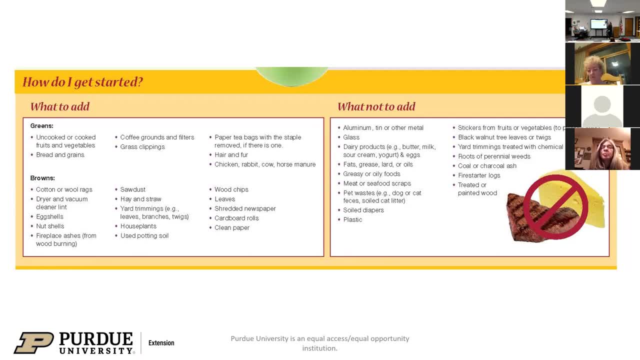 Yes, Lynn, I have. the way I've been composting was just a really simple way. I got three tubs that were like this deep an angle, So she's showing this about. yeah, Yeah, Like totes, Yeah. 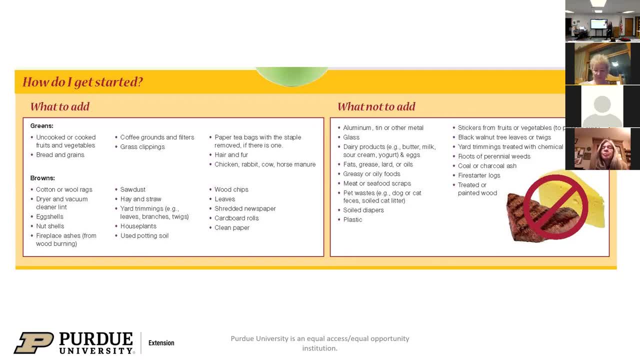 Totes pretty big And I just threw everything in there. They don't want to start smelling bad. That's when I put shredded paper in there, Okay, And I never had to add water or anything. And then, when the bottom was done, 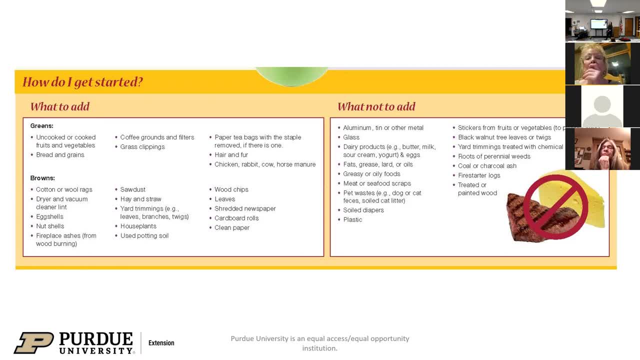 I don't want to mess up. the way it is, You do it here And when it's done you bring another one up. Oh, so you're doing three stacked? Yeah, Oh, I see As they go like this one's done. 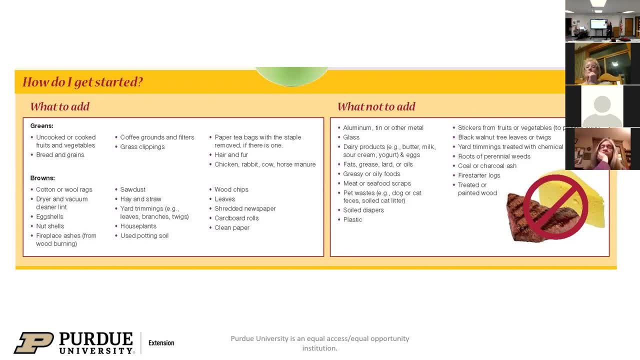 Yes, Now you start with this: Yep, Yep. That's what I did, And when it took me eight months, and when I emptied them out it was soil, I was amazed. That's awesome, I couldn't believe it. So she was showing that she basically had three totes kind of stacked within each other. 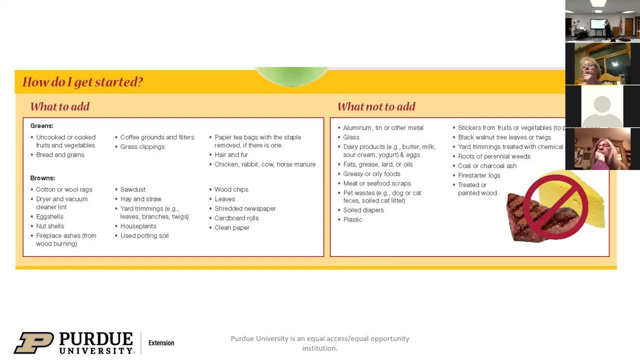 They had to be like this. They were like this So they could nest in each other, And you basically let it move its way down. So basically it was filtering itself almost to become soil. Yeah, That's so cool. I didn't do anything. 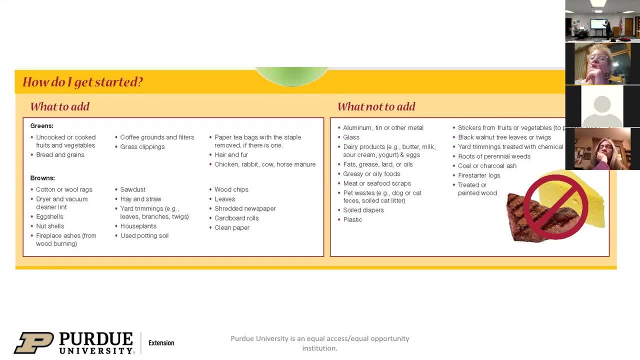 So what they suggest? If you're living in a neighborhood, obviously don't put metal or glass because it can hurt you, because you're going to be putting it on your soil eventually- Fats, grease, lard, oils, meat. Now, if you live in the country, you can do that because compost will eat your meat right. 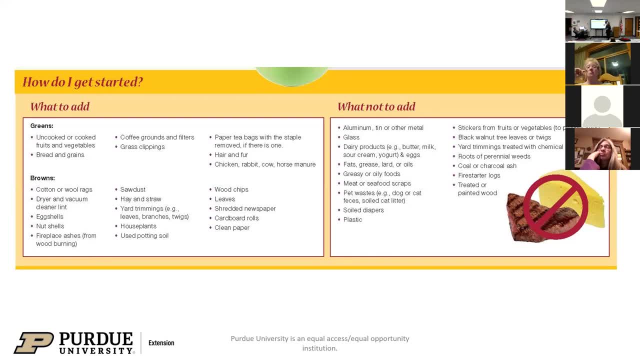 up Like it'll eat dead animals. That's an acceptable way to get rid of dead animals composting, But you have to make sure there's a fence around it so that your neighbor's dog can't come bother it and scare the neighbors. So, but compost will eat. You don't have to dig a six-foot hole because I don't know about you, I don't like digging six-feet holes when animals die, So it's a nice way. but you can put meat, but just you have to not let your dogs labor. 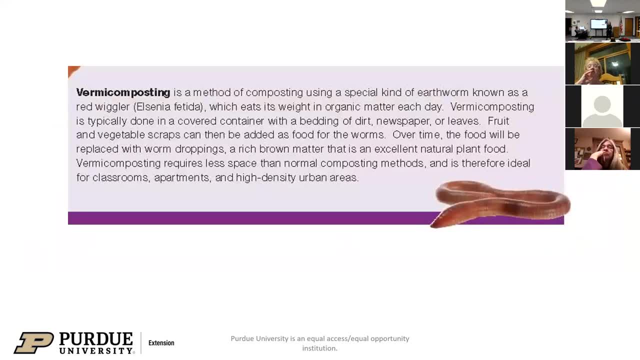 dogs get it, Okay. So what do you guys think about this? I vermicompost is earthworm castings, which is basically feeding your earthworms and they poo and pee And then they make an awesome cool either tea or they're castings, which is like a. 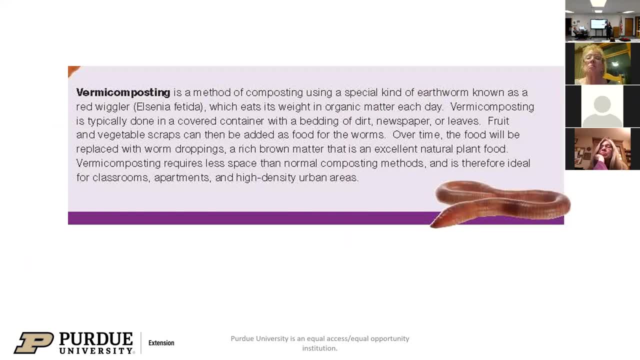 little bit like, looks like soil. vermicompost is something. I was thinking about buying a vermicomposter so we could show people here, maybe kids, And so it'd be part of my programming. What do you guys think? Do you think that's a good idea to have that and talk about it and show it? 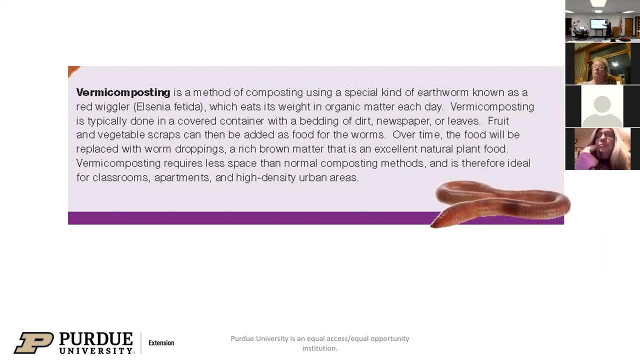 Okay, cool, I'm going to buy it. I'm going to totally buy it. So basically, vermicompost obviously takes less space and it's kind of cool. There's specific types of worms, but any worm would work. But red wigglers work mostly really well in a vermicompost system. 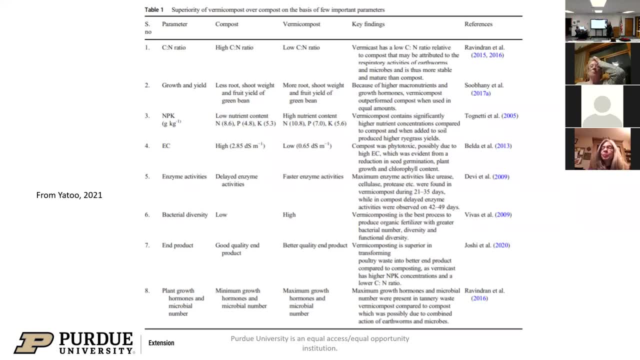 So I think this was really neat. Some research has been done about what vermicompost is good for, And what they found is they actually find with here's, compost on the left and vermicompost on the right. You can't see it, because it's right here. 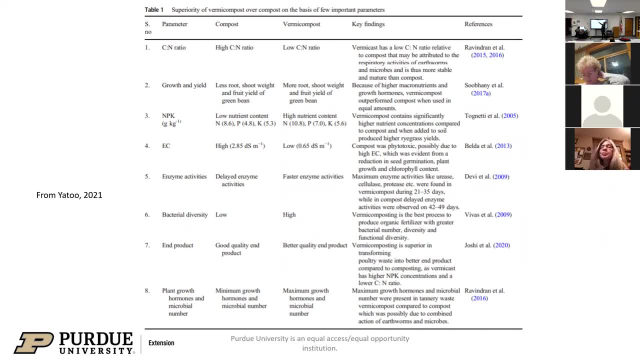 Basically it shows the different carbon to nitrogen ratio. So basically there's a low carbon to nitrogen ratio for vermicompost. That means it's very high in fertilizer. It gives Plants more roots, shoot weight and fruit yield and green beans. 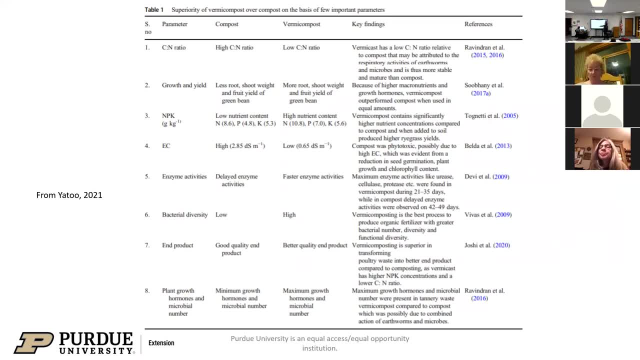 So they did this research to show you what vermicompost does. What I think is very interesting: eventually better quality end product for gardening and its maximum growth of hormones and microbial members with vermicompost. I think there's another section next, because it actually keeps diseases away. 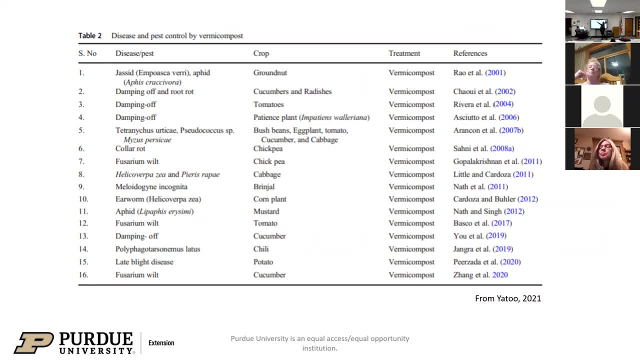 Yes, so they had some diseases and pest control by vermicompost. So look at the disease: pests like aphids In the ground that I don't even know the ground, that is but something, and vermicompost helped it with those aphids. Basically there's less less aphids on that than it was with without vermicompost. So it helps with dampen off and root rot and cucumbers and radishes. It helps with dampen off with tomatoes. Who knows what dampen off means. 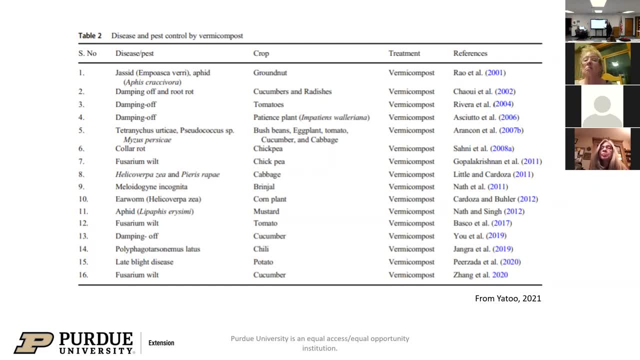 Yes, Mike, what is it? Don't ask me to explain. Okay, Have you ever had it happen? I don't want to know. I'm trying to do this easily. I'm trying to do this easily. I'm trying to do this easily. 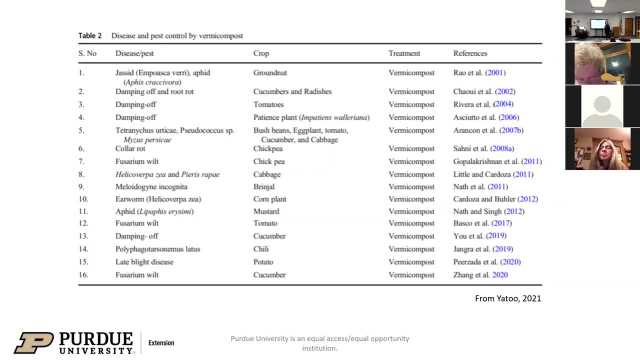 What does it look like when it starts dampening off? When you have your seedling and you have it inside and you're so happy. It gets that black part of the bottom and just gets. so it dampens off because it's a type of fungus. 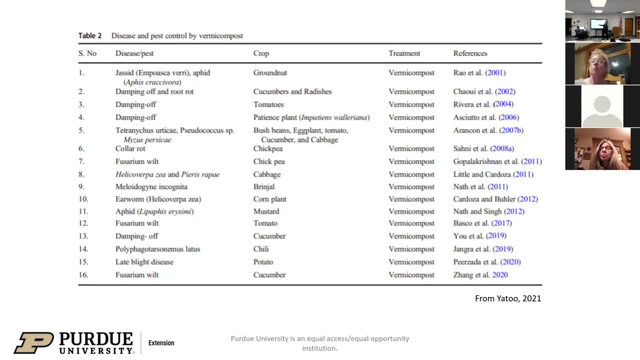 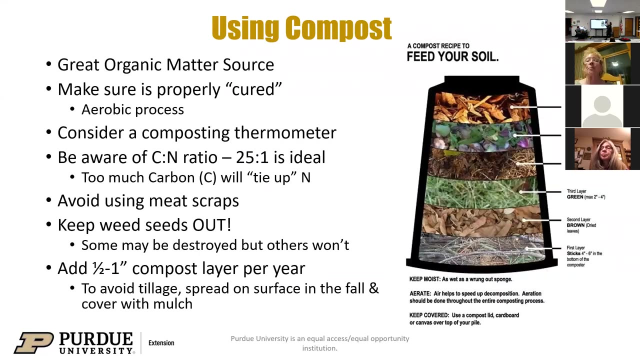 But tomatoes are helped using vermicompost from dampen off, So it's very interesting. This is kind of unclear why, but basically it helps to prevent pathogens and pests, which I think is interesting. Go ahead Basically using compost, feed your soil. 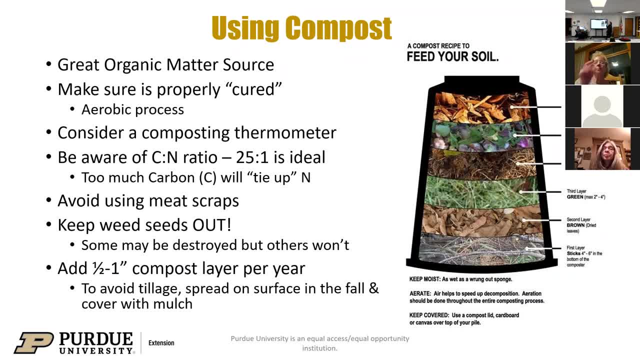 So if you weed seeds out, just be safe and don't put meat in there for your neighbors And just kind of look for the carbon to nitrogen- about 25 carbon, which is about 25, like leaves and brown stuff- to one, nitrogen is about as a good amount. 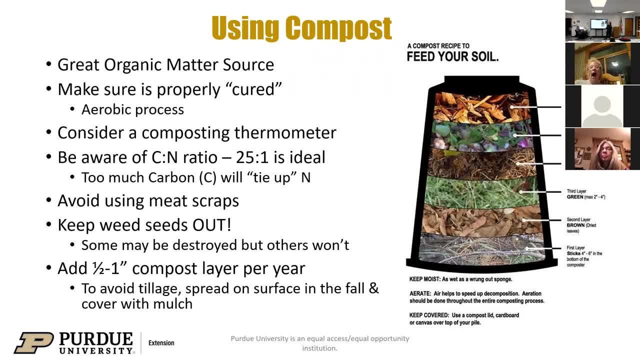 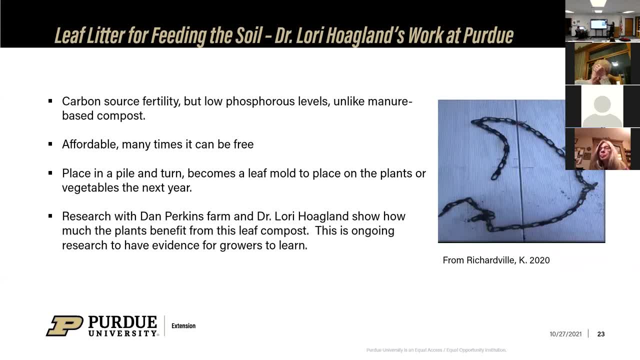 But you can't really go wrong. You're not going to mess it up if you put too much in one or the other. So here's really interesting Talk is: this is a chain that was actually found in some leaves. Have you ever seen when the downtown they put all their leaves out and they kind of suck them up? 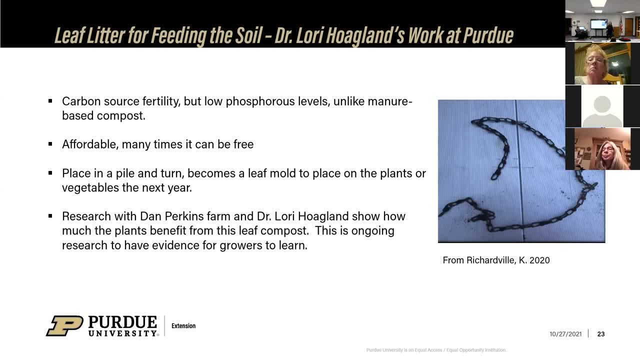 or they like put them in bags. Well, there's actually research of it, Purdue this farmer. it's called the Perkins Farm Farm. They live on sandy soil and they're doing compost research because they need compost for their sandy soils, all nutrients in. 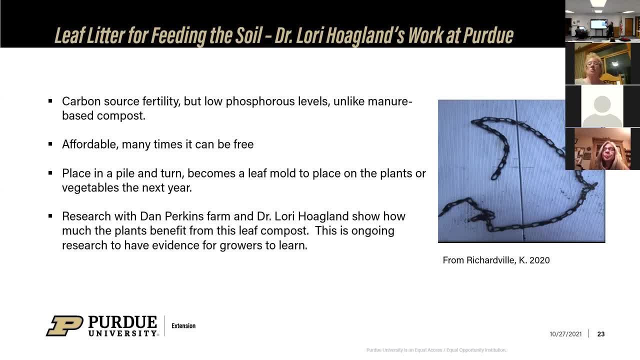 And they were given a lot of free bags of what leaves. Well, this was in this, this chain was in it, And that's not a good way to get your iron in plants, is it No? but so you got to be careful getting too many leaves from municipal sources. 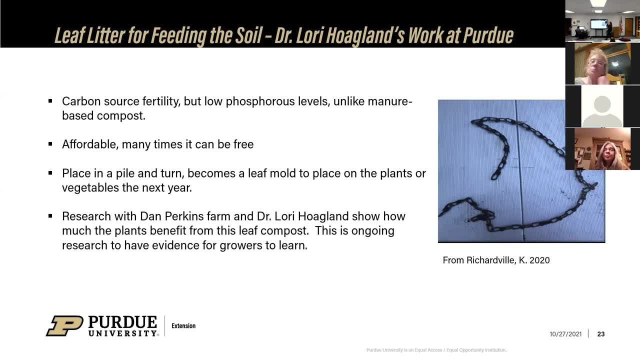 There might be junk in there. So you got to know that there is a risk And also you need to probably test it, because there could be salt in it from the road which can actually affect your plants. So don't go too crazy on it without testing it, because you don't want your plants. 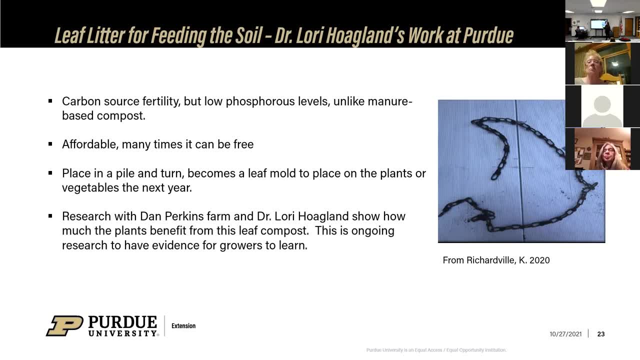 to not grow next spring when you put them on there. Many times, Though, have you noticed, leaves are free. lots of times, People don't realize the goal that they're sitting on, and they just take it away. It's you just basically so easy to put in a pile and you can turn. it. 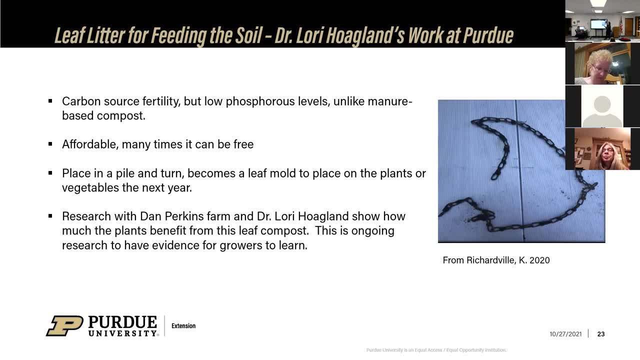 if you want, or just leave it there and it's going to turn into compost. And research with the Perkins Farm and Dr Roy Hoagland- and she's actually written an article that should be coming out soon in a journal- Show how much the plants benefit from this leaf compost. 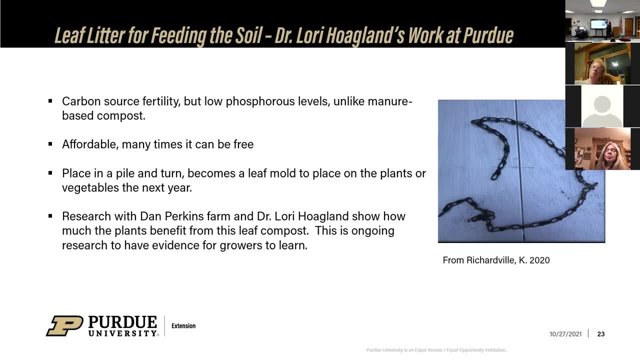 We're going to show you some pictures from the research that she allowed me to share, which I think is really So. what happens to the salt once it eats up? That's the hard part. I don't think it goes away, but I think microbes could help it. 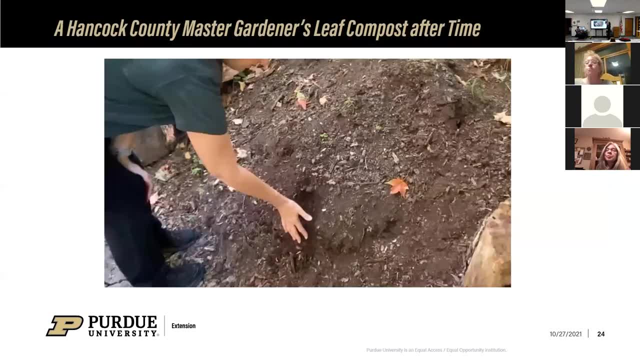 So you've got to be careful. You know what I mean, But you have to be careful too with herbicides, like when you have it untreated. I don't know how long you're supposed to wait, That's true, But I know I will put it in my compost pile. for months, several months after thinking about it. So I'm going to put it in my compost pile for months, several months after thinking about it. So I'm going to put it in my compost pile for months, several months after thinking about it. 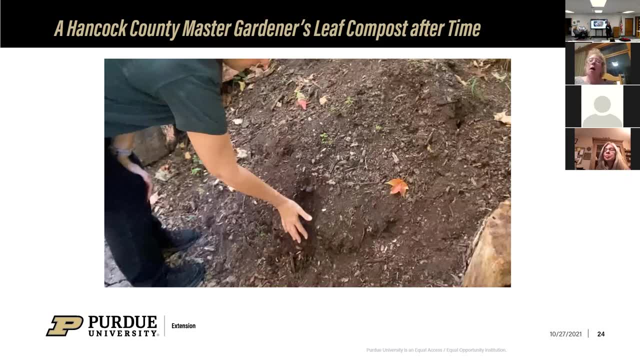 So I'm going to put it in my compost pile for months, several months after thinking about it, But so you know you're what's treated on your yard. Is that what you mean? Yes, Yeah, You have to be careful with that. 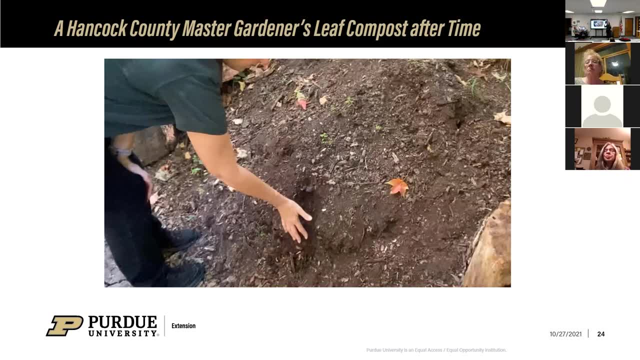 That's true, And watch out for horse manure, that sometimes they- actually horses, are given a type of hay that keeps them from having weed seeds. I get kind of confused. It's a type of herbicide in their feed or pesticide that can actually get into their manure. 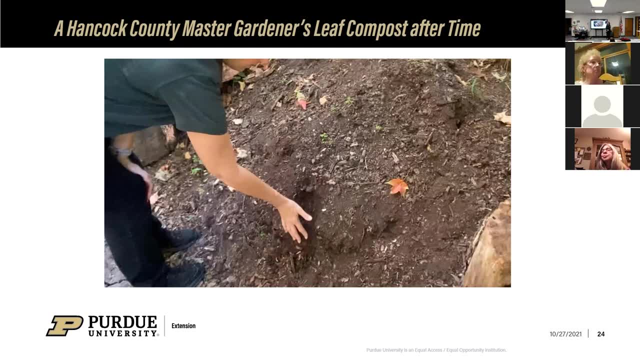 and stay there for a really long time. It's a long residual for that. Yes, Glenn, I just had the vet out because of one of my horses and he said that GMO affects horses' lifespan. Oh, I didn't know that. 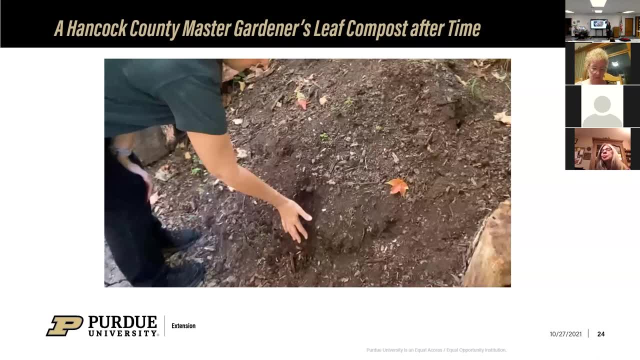 And GMO stands for genetically modified organisms. Right, He's found with the study that he's doing that he has Cushing's- that the GMO and the spraying of pesticides and so on and so forth is affecting the pastures where they eat and it affects their health. 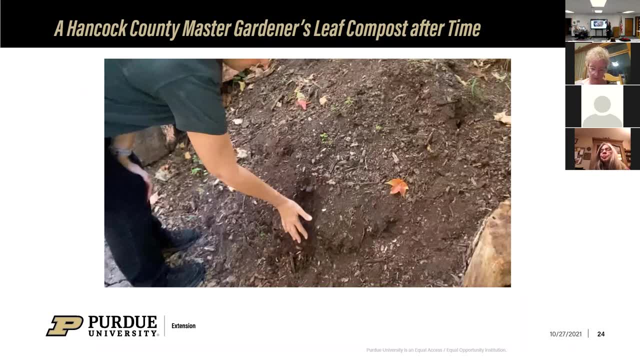 He thinks that's what's causing Cushing's And Cushing's is swelling up the house. It's a tumor, Okay, Yeah. So he's trying to get him off the medication. I put him on organic feed, which doesn't have any of that in it, and limit his time on grass. 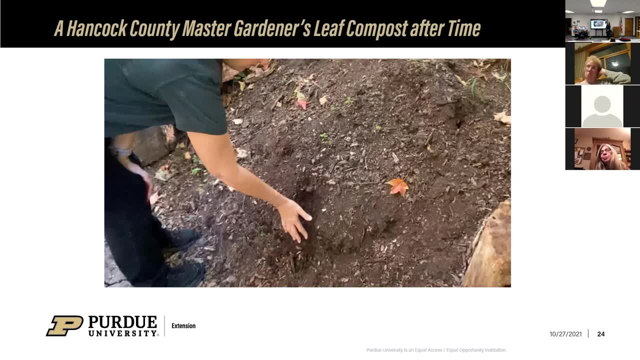 And he says we may be able to get him off the medicine. I said, wow, Good Thanks for sharing that. That's good. This is Marianne's leaf compost going leaves and basically you run over it with your mower. 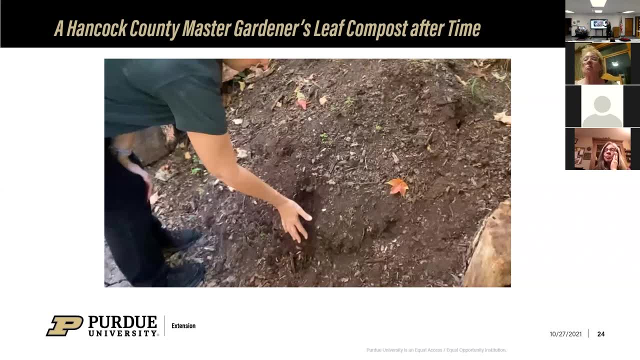 a couple times and put it over here. Now we have a machine that looks like a grinder. We just sweep it into this mulcher and we just like we'll spend a couple days, total solid days- of just raking them into this thing and spreading it out, and then it just 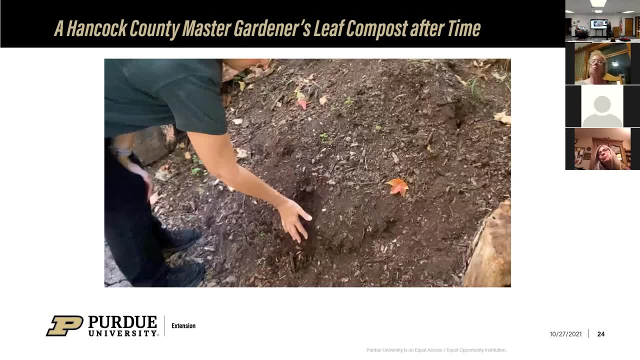 sits there all day, And so then we throw in the spring the grass clippings in the kitchen and then it sits there. So that's probably from the year before. Yeah, It just sat there, So it looks like dirt. 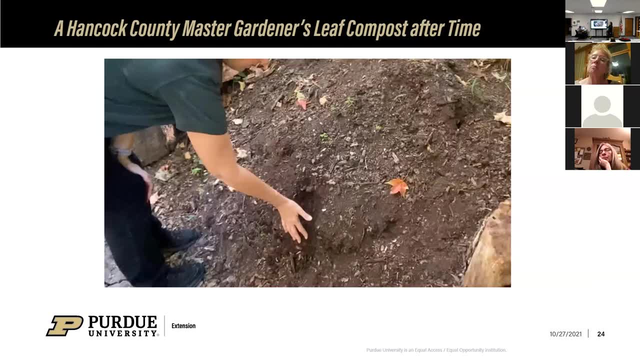 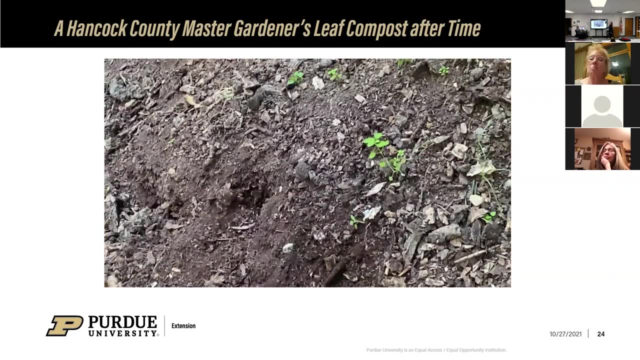 Yeah, Go ahead and push the video and maybe we'll see how much it looks like soil. See what works? Yeah, they are. That's just leaves. That's my compost. Yeah, Yeah, Go ahead, Go ahead. Thanks, Marianne. 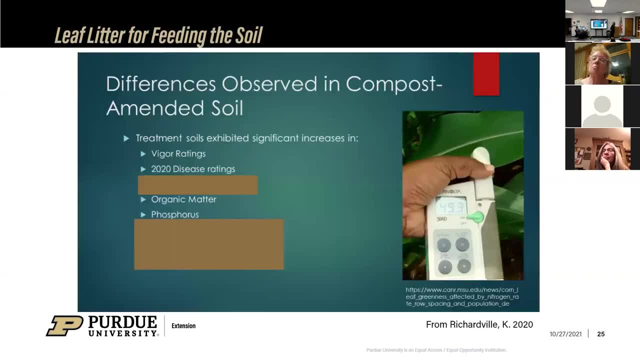 That was an awesome demonstration. It's a huge pile too. This is differences observed. Oh, go ahead. Does someone have a question for me? Yes, Marianne, I'm getting a little confused on when do I put the compost in. 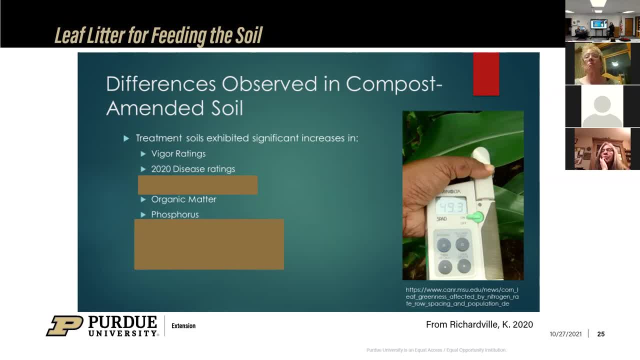 It's like I'm getting my garden ready. Yeah Well, you have leaves now, right, So start a compost pile with your leaves. Oh no, no, I've got compost. Yeah, I've got to add just some regular soil to it. 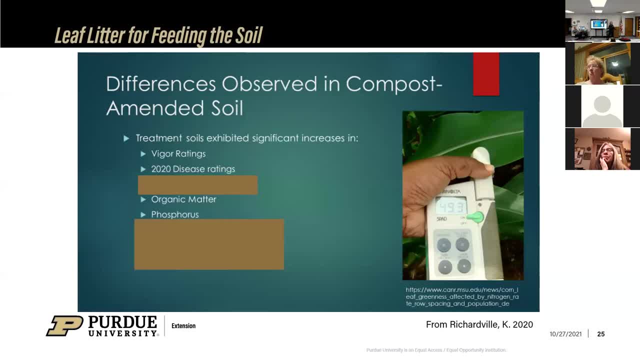 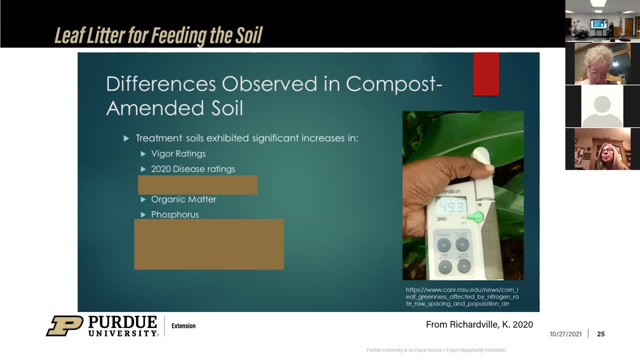 Yeah, And do you plant a cover crop now and wait and compost it in spring? Actually, I put the compost on in the spring but I don't dig it in. That's fine. I find that when you try to make it real pretty for the plant and then critters come and get. 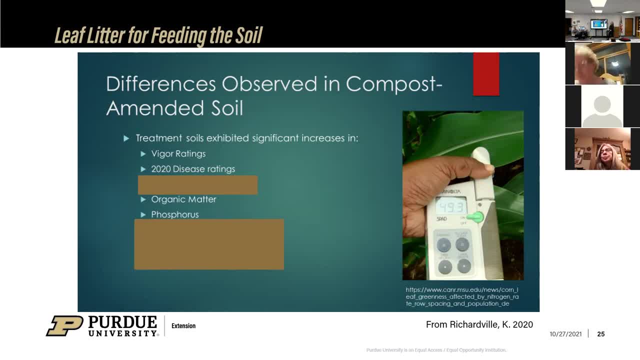 in there And so basically, and I, actually I spend some time volunteering at the Museum of Art. It was a very, very good. That's exactly where Bruce works too. Yeah, Yeah, I'm Facebook friends with Bruce. Oh, you're working with him. 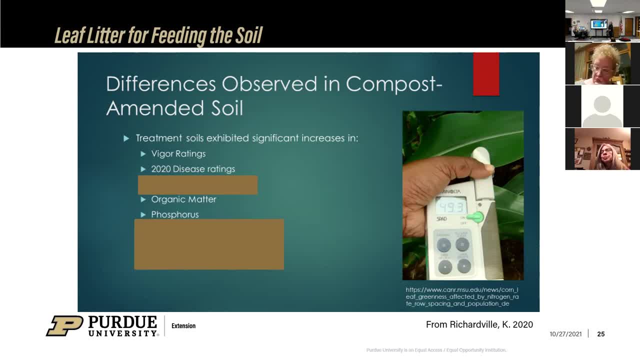 forever with patty, and so basically, she basically just kind of taught me a whole lot of things and one of them was: don't dig it in, just spread it on top, and it really does absorb and take up the nutrients in the soil. and you could, if you already have compost ready, you could- put it on in the 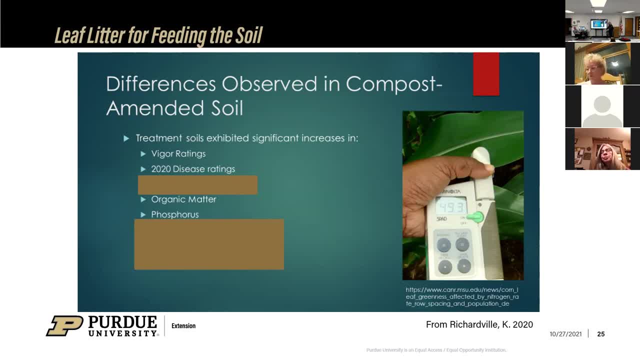 winter it won't hurt at all because it'll take the time to get established in soil. but you really can't go wrong once you have compost, except don't put too much- about one to two inches at most. the reason i say that is sometimes too much again can be overwhelming to the soil you don't want to. 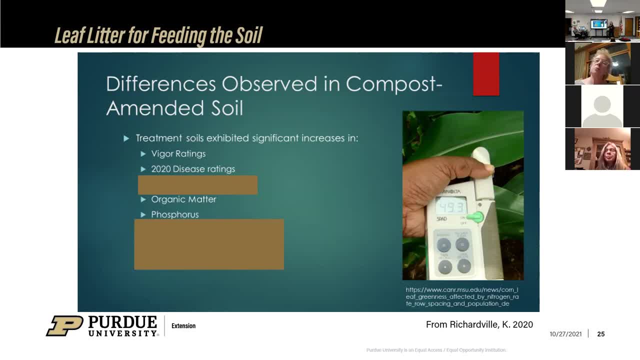 overwhelm it. so we get so excited. we want to put like six inches. that can actually cause problems, so don't go too excited about it, but you can put it on now if you want, or spring. well, that's what i was told is that you only do it once a year? yeah, but so that's why that's all sitting there. 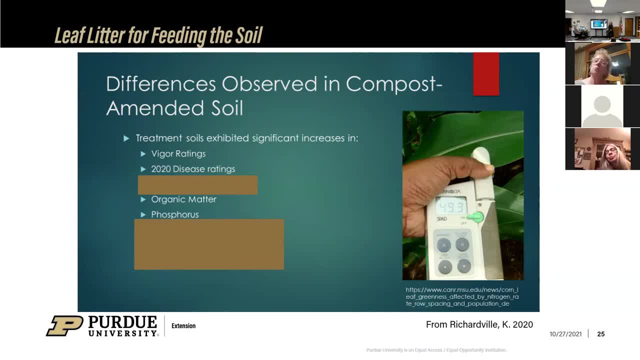 because it's waiting for the next season, because once i spread it out, then i'm kind of done now, but i don't ever go do something. basically, it's it's weight and you kind of have to be patient because, um, you want to go, you know, spread it more again. but but it's more fun to work in the winter personally, because it's. 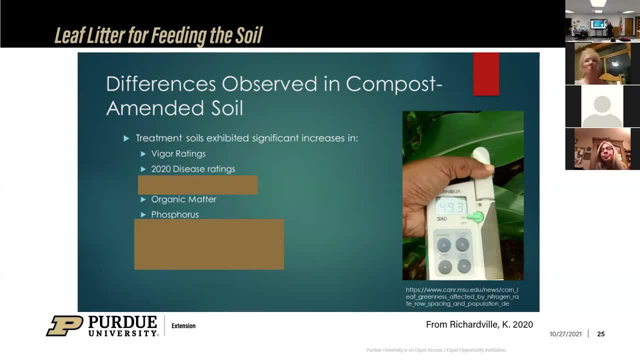 cooler, so every fall. but so the reason why people say once a year is just because mostly we do all we work in spring, because we're excited. but it doesn't have to be like that. we just once a year, right. yes, you don't have to. there's a lot of benefit in putting it on in the fall, where you 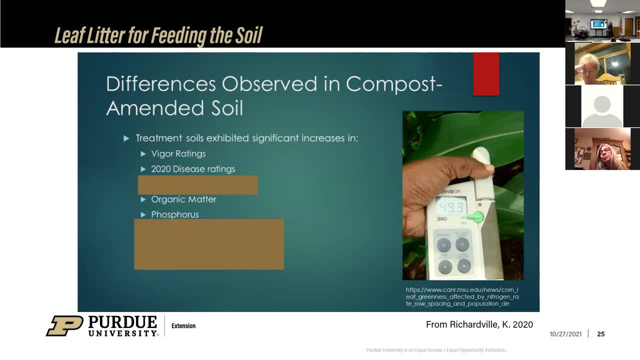 get snow, yes, and actually microbes live in the winter also. they're alive, they're not like dead. they need something in the winter also. they're more quiet and they're not as active, but they would be happy to have your compost cover crop can help too. so now cover crops right now. an easy one was given to us that. 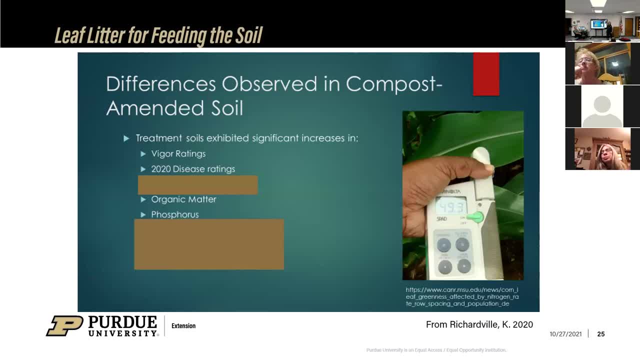 because they died the first frost. those are super simple but they won't come up right now. germination: probably you could still do rye, but that is really hard to terminate. they may need to find the same for that. it can be hard to terminate. clovers could work, yep, just kind of depends on your. 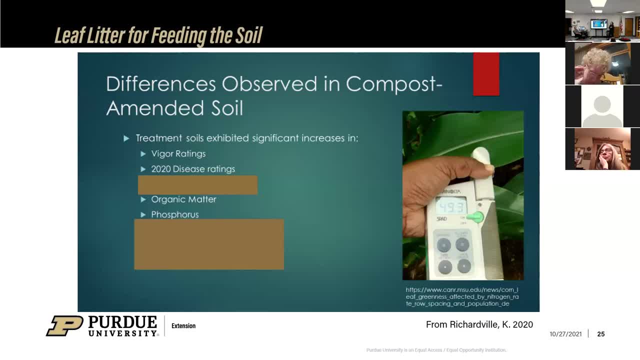 goals. and i don't know, the clovers would germinate. right now i'm not sure. i don't think they would only rye, i'm pretty sure germinates up until about 40 degrees. you could do barren hopes. turnips, radishes, the cold weather, cool weather, yeah, radishes. um, when they die, they do smell bad. 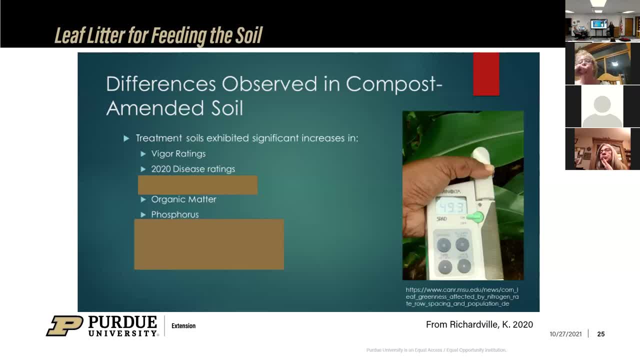 like especially the daikon radishes, but they will if you have a. if you want to cover it, you have. there are some options. just depends on how you want to kill it. winter wheat- yes, winter wheat, but it's not the easiest to kill either. i mean, you have to probably use a glyphosate or something. 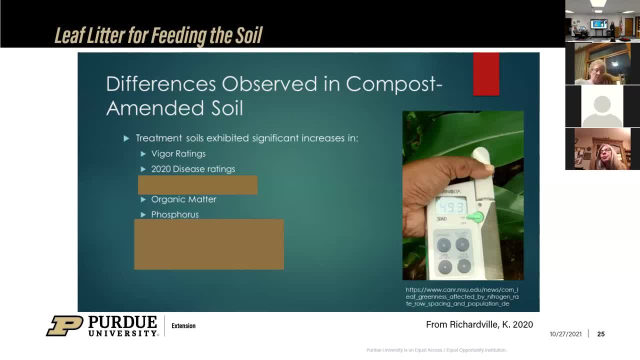 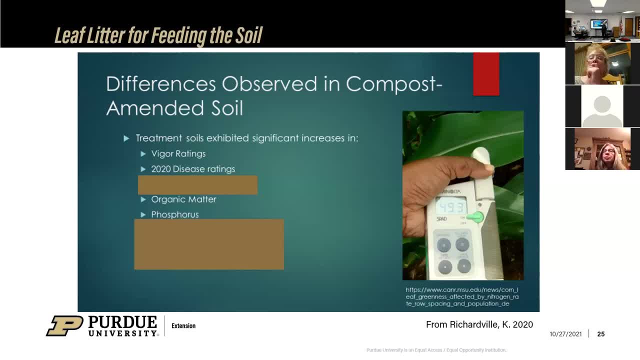 years. bigger ratings, which is how the plants grew. disease ratings: it was better in the ones that had compost. organic matter increased and phosphorus was the same in terms of it didn't increase with the leaf matter. i only covered these. it's not like they're censored, it's just i didn't want to talk. 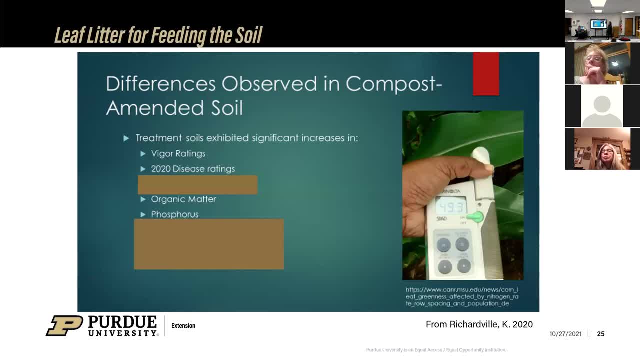 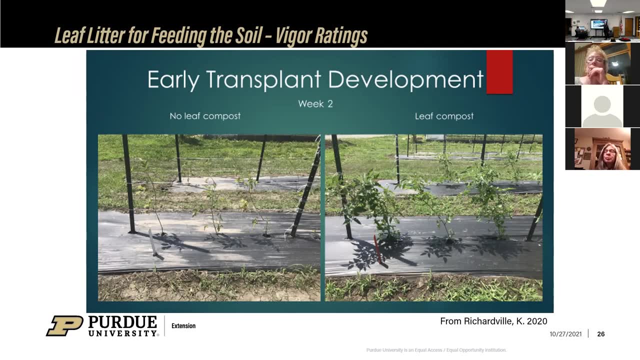 about it. it becomes too scientific and it's like overwhelming, so let's go ahead. so here's- here's a picture. on the left: no leaf compost. this is after two weeks of transplanting this, these tomatoes. on the right, they used leaf compost. that's the only difference they had. can you tell the difference? 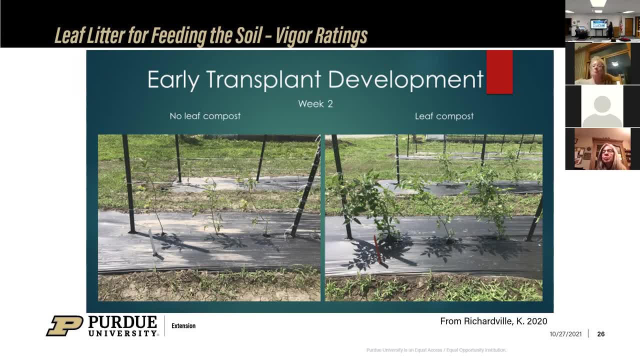 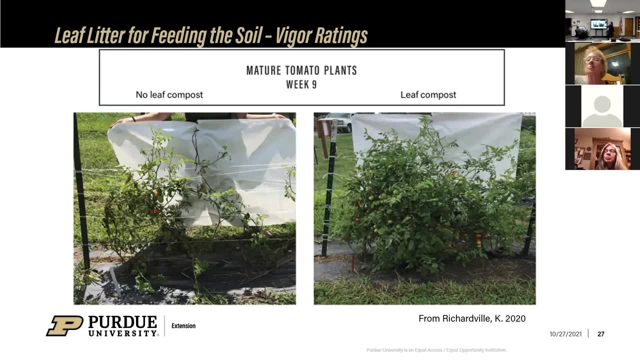 the one on the right obviously has stronger vigor, and all of it is this leaf compost added. go ahead, mom. then they did mature plants after week nine. on the left, no leaf compost. look at poor guy, he's all scraggly. and on the right plant, that's all the difference they had. 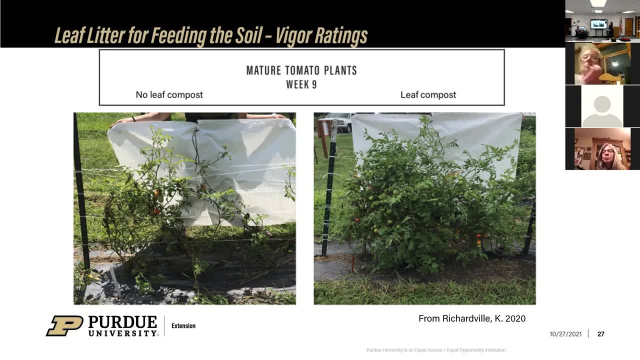 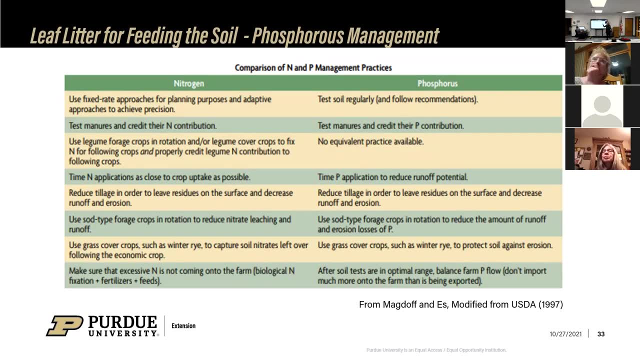 was leaf compost. go ahead. that's the bigger ratings looking at, just with our eyes. so phosphorus, phosphorus management- if you have too much phosphorus leaf matter is really important because, like i said, if you've gone crazy with animal manure, you may have too much phosphorus. 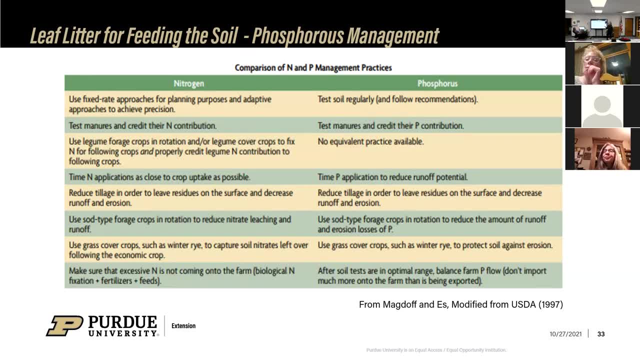 which could actually eventually cause your plants not to be uptake some micronutrients. you have to have a pretty high phosphorus, but you know you might, so just test your soil, and so that's. what's nice about this is that you don't have to have too much phosphorus. you don't have to have too much. 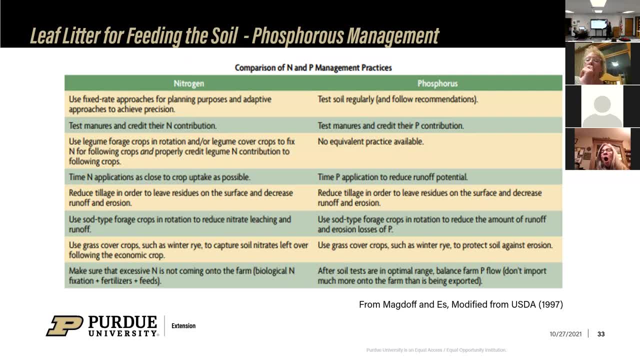 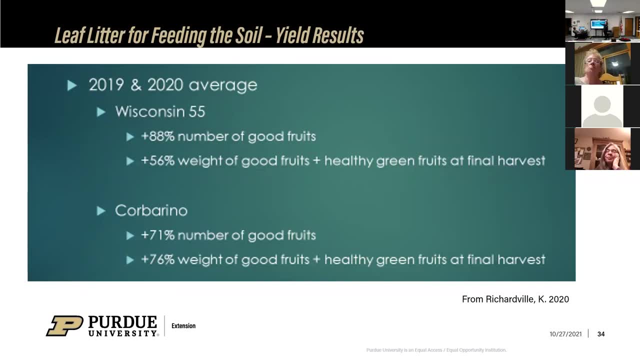 leaves is you're not adding more phosphorus to your soil. go ahead, thank you. thanks, you're georgia. yeah, georgia. this is cool. the yield results. so basically they're looking at 2019 and 2020 averages. there's different types of tomatoes. the top was called wisconsin 55 and the bottom is: 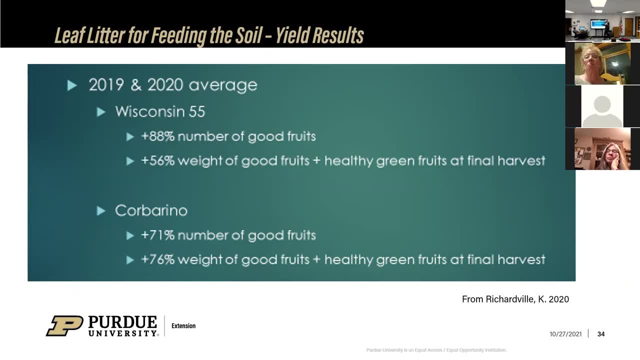 reno or yeah, whatever, and basically it showed with leaf compost it added 88 more good fruits and they were 56 more weight. so it's not just about the numbers, it's about how big those bad boys are. and then the bottom is- you can read it: 71, 76.. 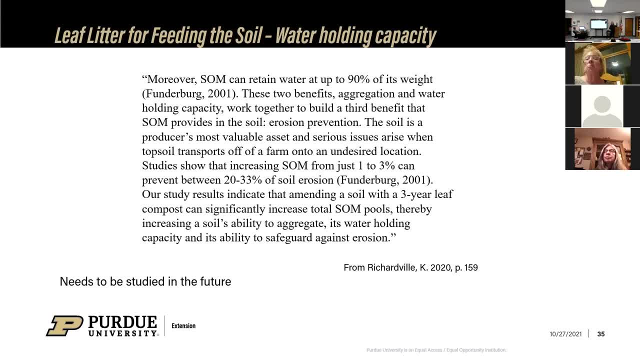 what's neat. how many have you had some flooding because of all the water recently? anyone flooding in your yard? yep, yep, yep, um, so we're only going to get more water in indiana. climate change is happening. um, we're talking about it more. we're talking about it more. we're talking about it more. 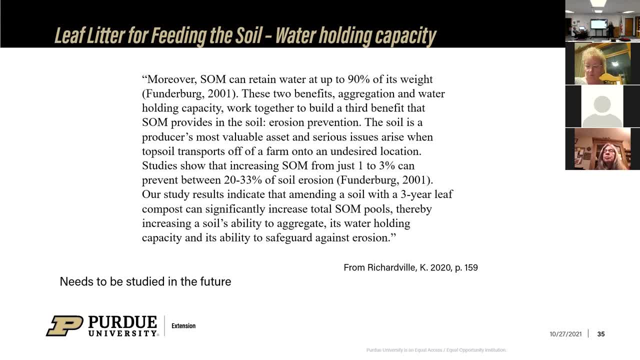 by the year 2050 we're going to be about our heat. we'll be able to have zone 8 plants. this is going to happen. i hope nothing happens really past that. it depends on our decisions now, because at the end of the century it works, but in indiana it doesn't mean all the states are the same. indiana we're 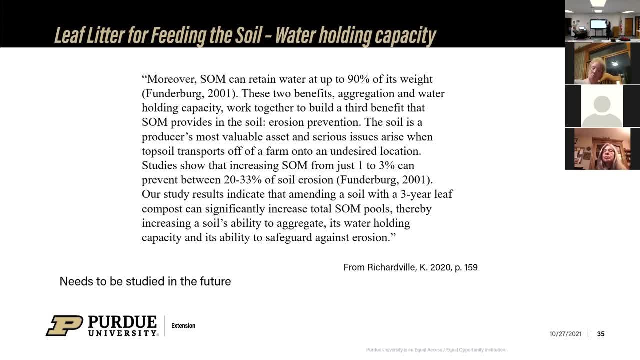 just going to be warmer and wetter and we're going to get more water and we're going to be basically having zone 8 planting and around our frosty of kentucky. so we're going to have longer growing seasons, which will be fun, and we'll be able to probably grow who mary is. that's going to be cool. 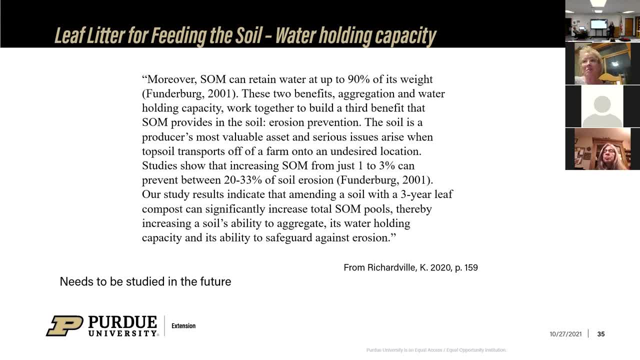 but we're going to have a lot more water and we already have a lot of water. that happens in spurts. so soil organic matter holds water and that soil organic matter is those microbes and those leaves. it can hold up to 90 of its weights. so imagine that leaf compost pile that marianne. 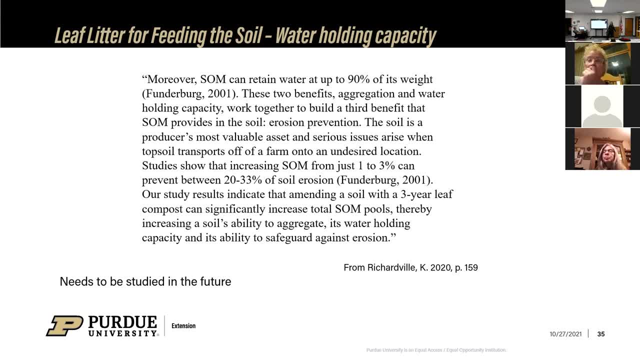 showed. that's probably. i don't know how many pounds that leaf is. leaves are right there. maybe 90 of its weight would be. you know, minus 500- i mean 50 would be 450- would hold that much water in that one place. i mean in theory. but the point is you want more water to be held in the soil and 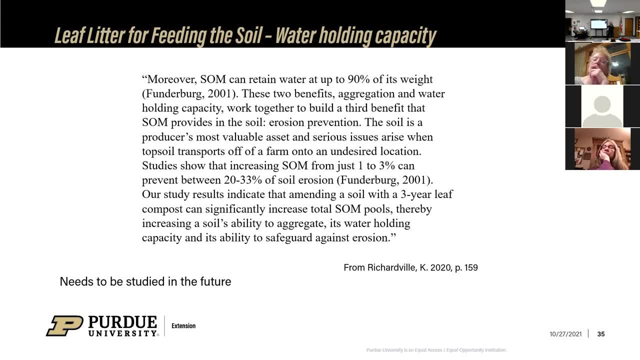 soil organic matter helps with that, but we don't want to go too crazy. there's a enough soil organic matter. about four percent is healthy. you don't want to go too crazy. yes, i do want to say it makes some difference in my house because i live on the hill. yes, and you probably don't lose it and i know. 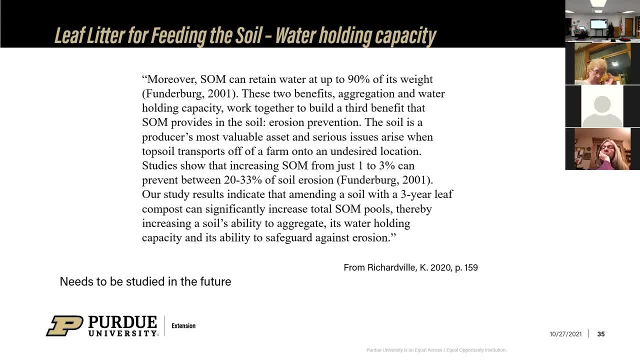 water, yes, yes. do you also not have to water? as often do you have to water your plants? i don't know. the only kind of time i ever water is a new plant. marianne says she doesn't have to water unless it's a new plant. so how many people would love to not learn this garden? i would, yes, because, first of all, if 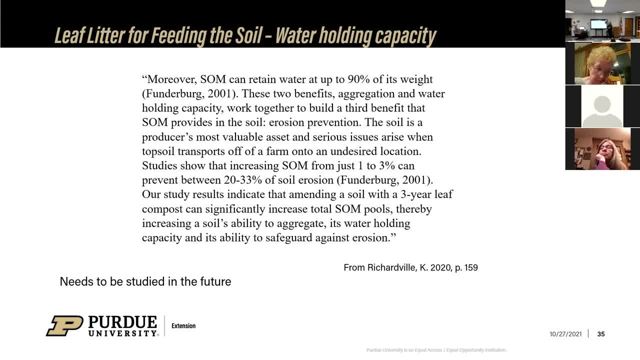 you live in the city. it costs money for water and it's really going up and obviously it's not work. so who wants to do that? so, basically, using compost or growing your soil, organic matter through whatever you want to do, mulching or whatever is going to hold the water, and those plants will be happier in the droughty summers. 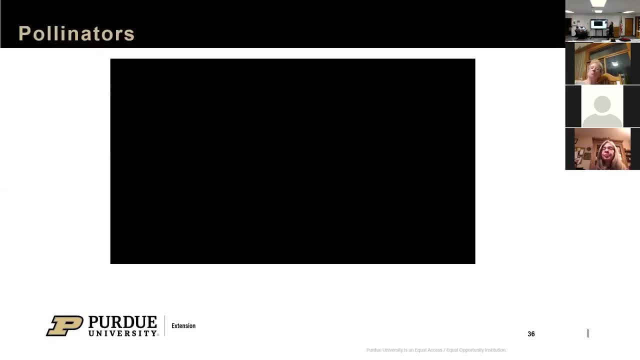 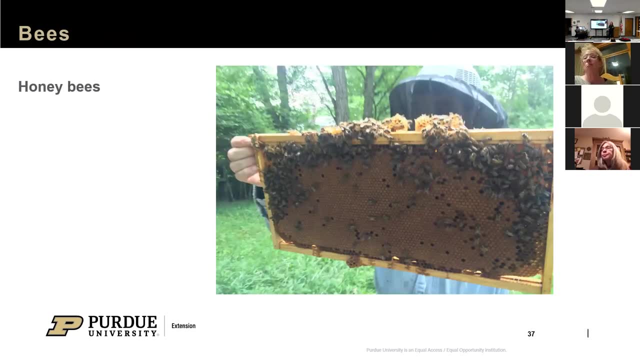 go ahead. oh pollinators, give them the next ones. so we're going to talk about why pollinators are important. here's my honeybees. honeybees are not native, they're actually called invasive. when i first heard that, i was so sad- i keep honeybees and i thought: oh man, that hurts my feelings. 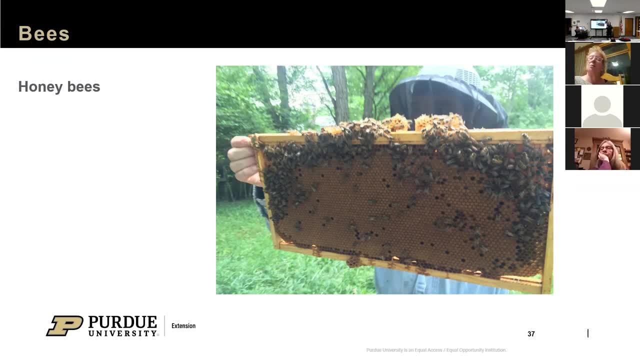 but actually bees are also good because we can do experiments on them to know what other pollinators are dealing with. but bees are generalist eaters. so if we don't have our specific foods for our specialist bees, the honeybees will just eat all their food. 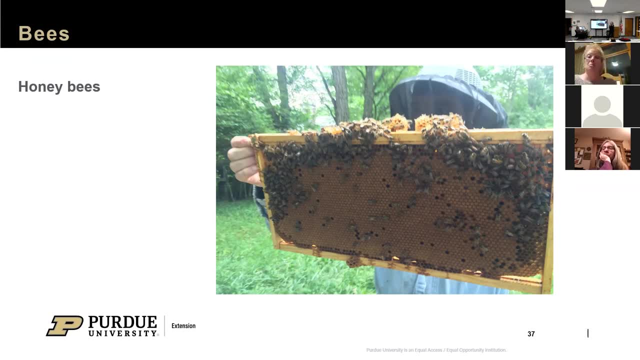 because they can eat almost anything, whereas specialist bees we have, like so many hundreds of kinds of bees in indiana, but they only live like within 300 yards of where they're where they're hatched and they only eat certain foods. so we need to think about those special speeds. it's. 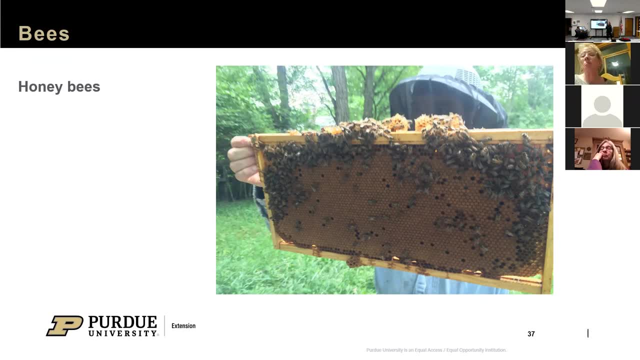 ok for a specialist bee that do the majority of orchard pollinating for apples, because they come out at 40 degrees, these orchard bees, but we give the honeybees credit because there's more of them that come out at 50 degrees. but those orchards are getting a lot of benefit from. 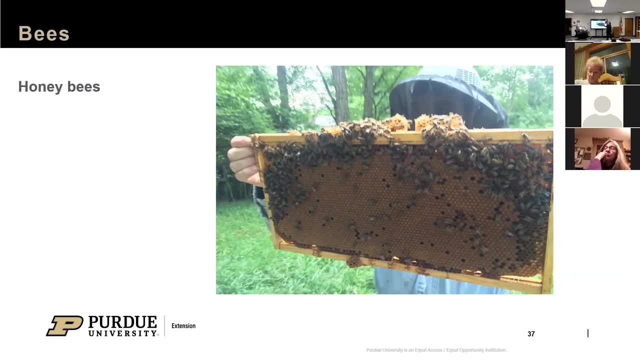 our natural bees, so we just don't see them because they're solitary, they live alone. they don't live in huge hives, and these are the more the they get the accolades, but really it's the our specific bees are getting a lot of the water. 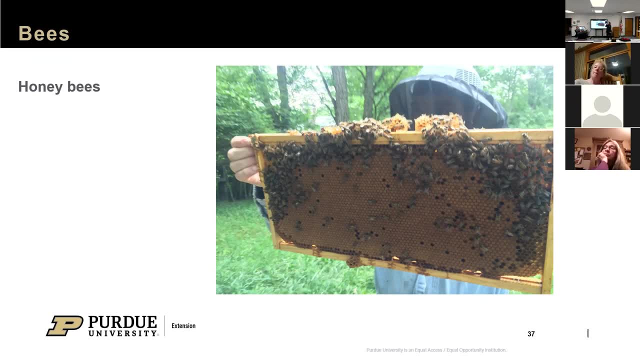 So do the orchards try to have those kinds of bees. That's right. There's no hive for them. They're learning that planting diversity around an orchard or any kind of place that needs pollination, like a pumpkin patch. it's actually more beneficial to have diversity around that. 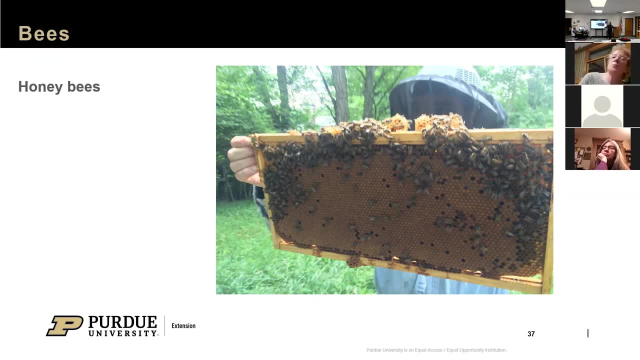 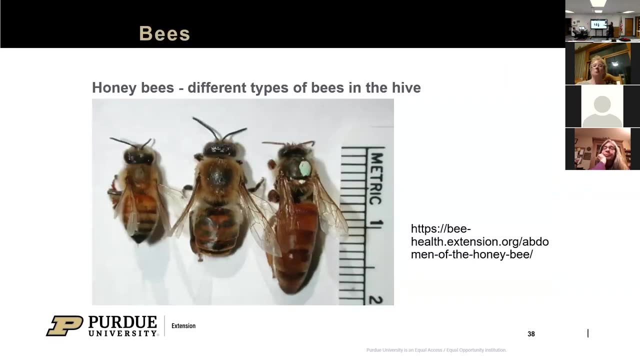 than to have honeybees, Because you're basically growing your specific bees around you. Yes, Isn't that interesting? It just shows different types of honeybees, And that's kind of the way it is with solitary bees. But again, they're solitary, They live alone. 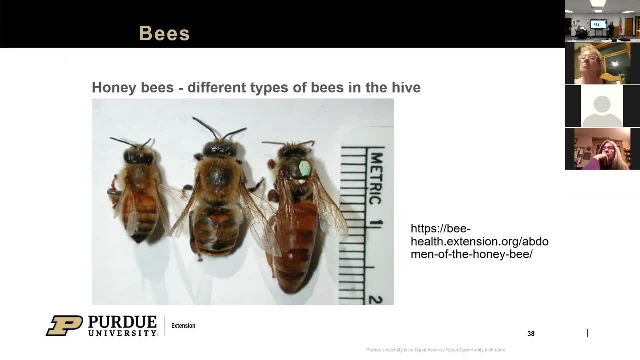 And you know where they're living. They're laying eggs in the ground. They're going to be laying eggs in stems that are left over. They're going to be laying eggs in parts of wood that you just have kind of on the side of your yard. 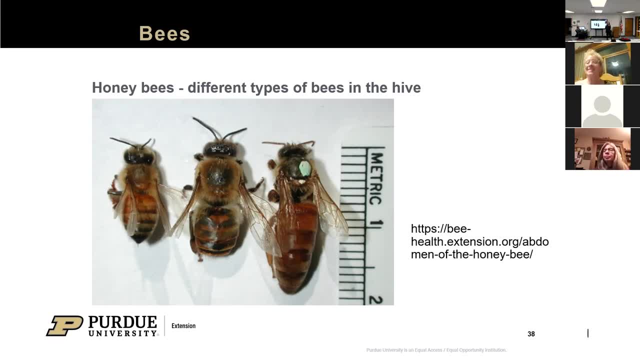 So having kind of a messy yard- in some places it's allowed- is actually good for your pollinators. Do you have an example of a solitary bee? Yes, Yellow jackets are very solitary, No, no, those are wasps. Those are a type of wasp. 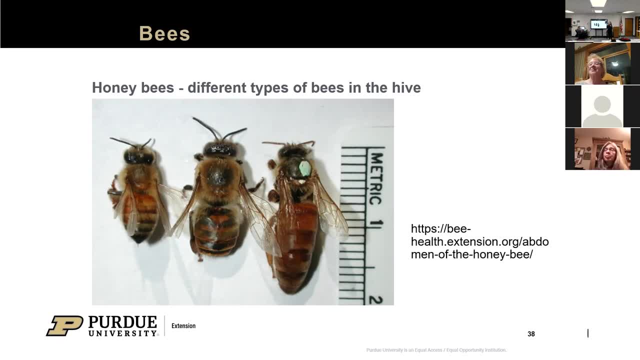 So a solitary bee is a leaf cutter bee. They're the ones that make like little holes in your leaves and they go to make their little nests And they're just pollinating things that we don't even know exactly what they're pollinating. 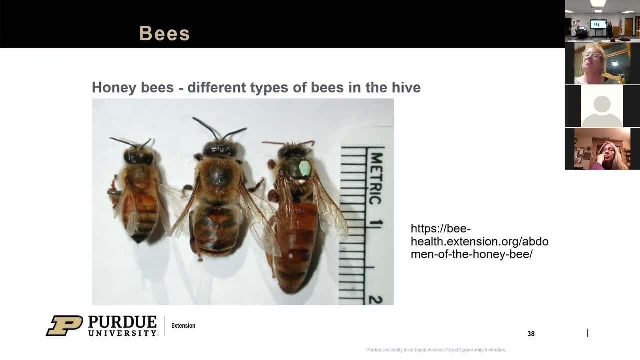 But they are a special solitary bee. Yep, Bumblebees, You see bumblebees all the time, Our asters out here. they're a solitary bee, I mean well, they have small homes, but they have very small amounts of bees. 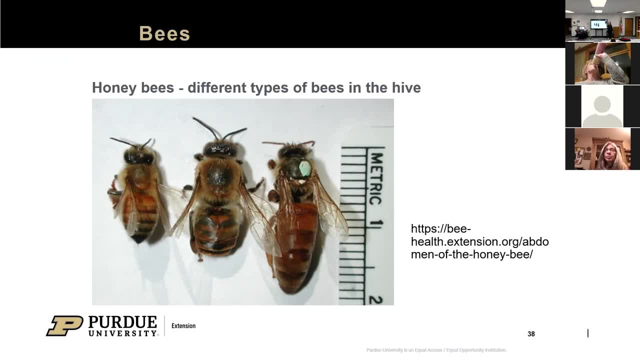 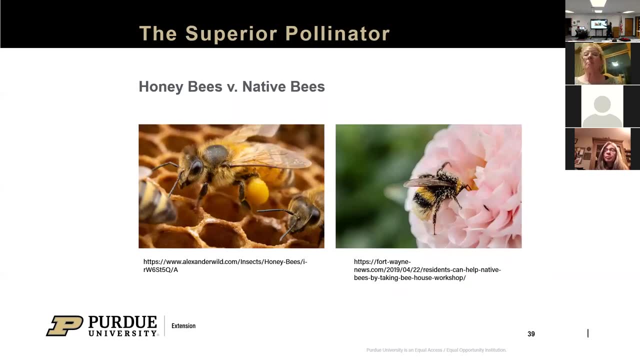 compared to honeybees, And the queen will only live over the winter. She's the only one who lives. Go ahead, Bob. Which one do you think is a superior pollinator? We give honeybees all the credit. You see what they're doing. 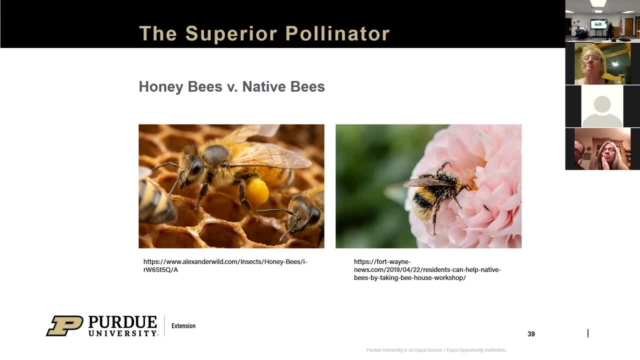 This is their pollen basket on the left. She's shoved that so tight there's not much pollen coming. But what is this bumblebee doing? It's covered. It's not holding it all tight. So which one do you think is the more superior pollinator? 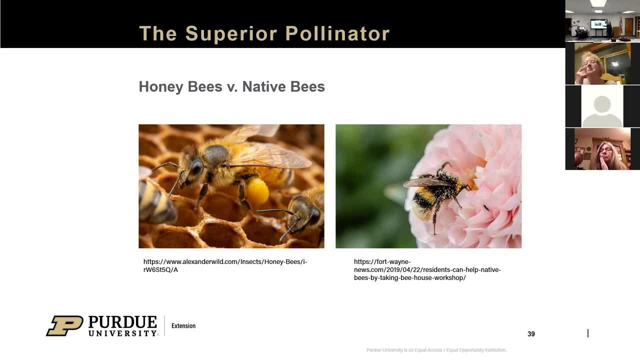 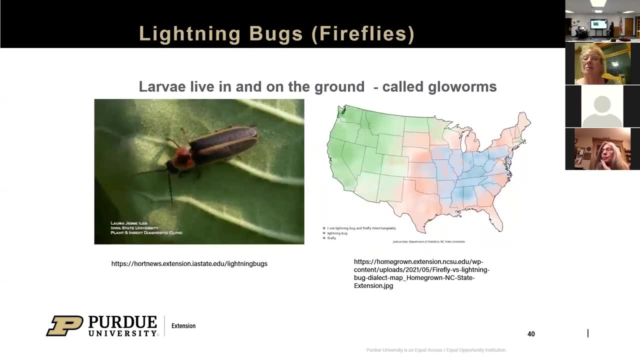 On the right Because she's accidentally just going to pollinate anything she comes in contact with. Yes, Lightning bugs. How many people have seen less lightning bugs since they were younger? Yes, Do you call them Lightning bugs or do you call them fireflies? 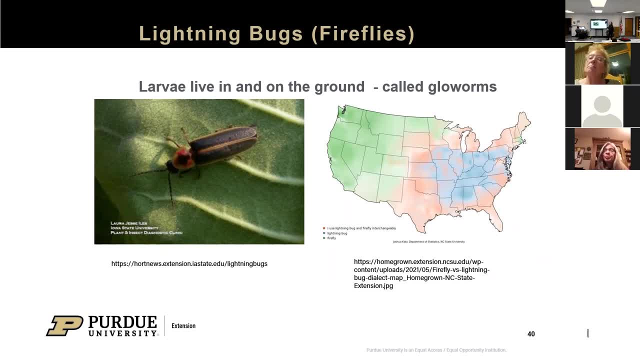 Well, people sometimes call them fireflies. And you know what? their baby, like their larva, is called Glowworms. Yes, And guess where they live? They live in the ground and right on top of the ground, right underneath the leaves. 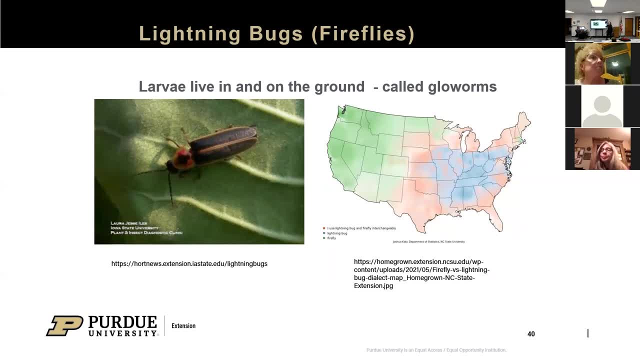 That's how they live over the winter. Sometimes they take about two years to become lightning bugs. But if you're killing grubs in your yard, you're killing lightning bug glowworms also. So be careful, Don't just willy nilly throw out your grub control. 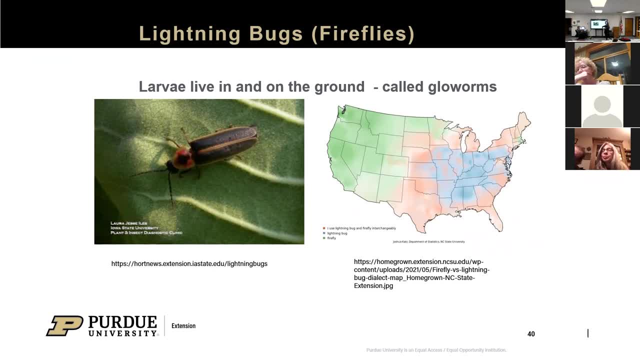 and think about maybe having a space over there for your lightning bugs, Maybe putting some leaves over there in a place that your neighbors won't see, and you may see lightning bugs come next year. So just think about their pollinators also. Lightning bugs are actually a pollinator. 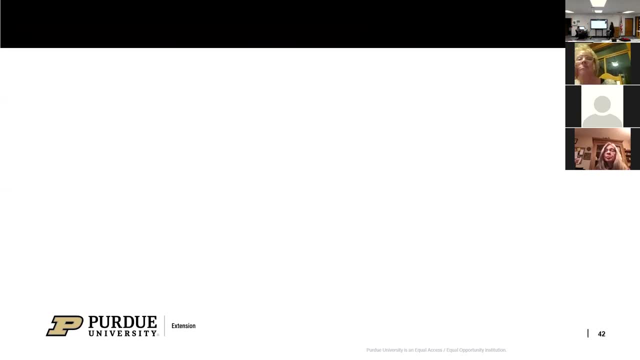 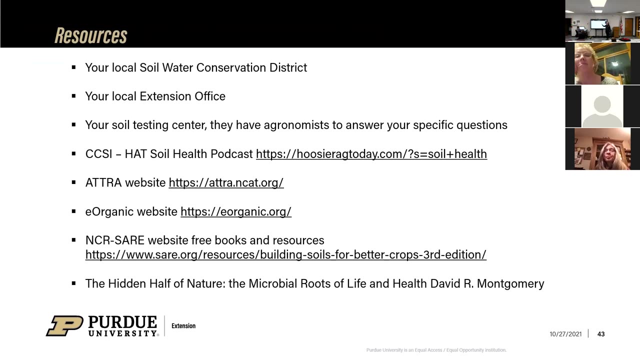 Go ahead, You can go to the next one. It's kind of boring, That one's really boring. That's really boring, isn't it? Yeah, Resources, Resources, Talk to Soil and Water Conservation District. They're all about pollinators. 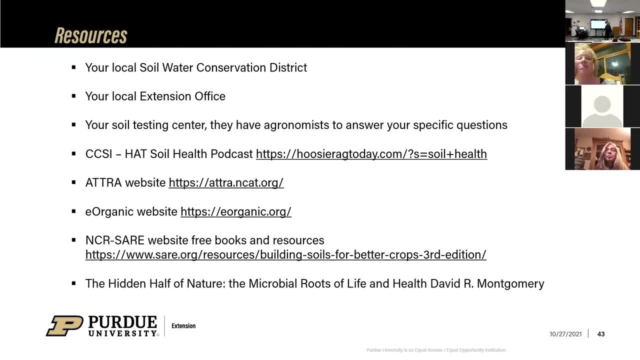 In fact, the NRCS wants you to grow pollinator patches. If you have a large property- I don't know how many acres, it begins to be about half acre- they will help fund it. They may give you a part of the loan. 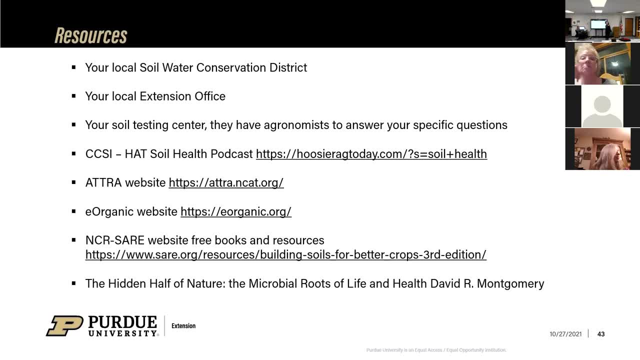 I'm not really sure, but you talk to our FSA, which is Farm Service Agency, and our NRCS, which is right down the road at 40, and you might be able to get some money to plant a pollinator yard acre. 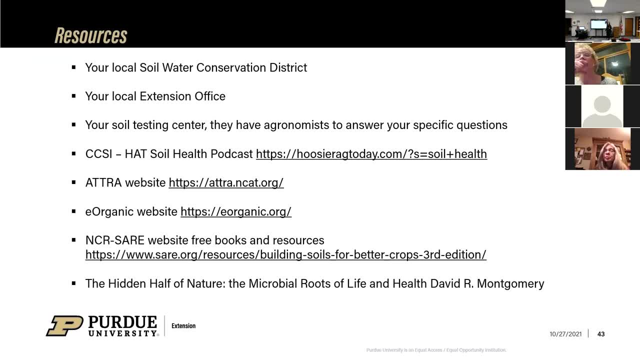 Half acre, whatever it is. So talk to them, because they know how important pollinators are, And definitely get your soil tested if you haven't already, And that's pretty much good. That's good. Anybody have any questions? 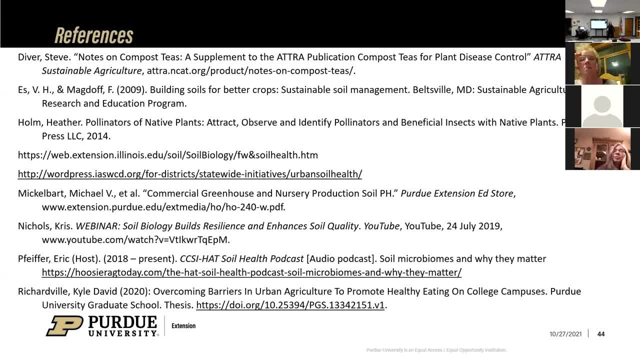 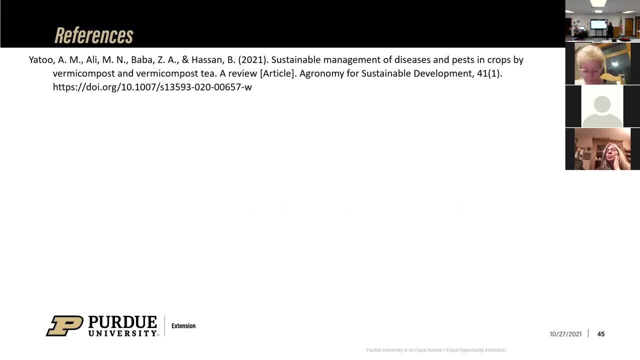 I do. Yes, Bob and I were talking Saturday about the gray piles of whatever in farmer's fields and Bob said he thought it was lime and we said, boy, that's the wrong direction. Why would they? Why would they be liming their field? 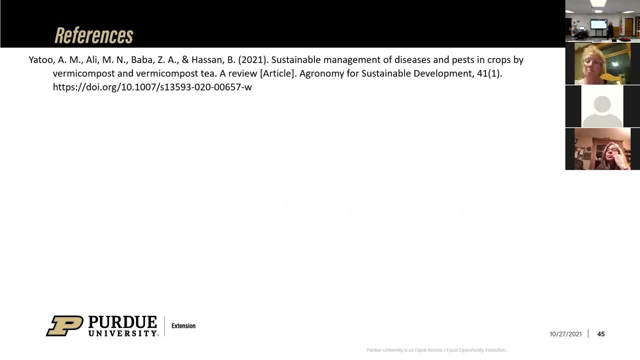 and reducing the pH. Do you have an answer to that? Well, I don't know their soil test. Hopefully they're testing. They're based on soil tests. Yeah, they wouldn't be wasting inputs if they didn't need it. It could be a fertilizer. 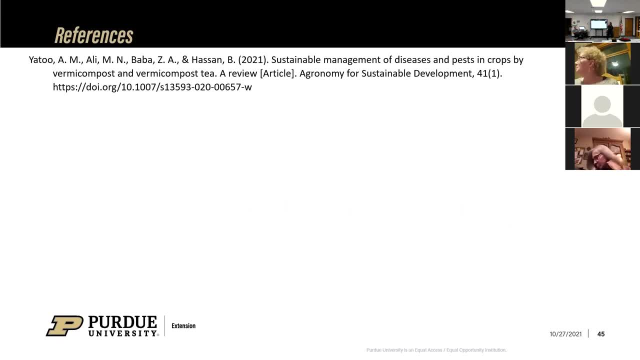 but a lot of times, most of them- I don't farm physically. I help farm and have for years- About every third year they'll lime to help loosen the soil. That's what they said. They're trying to loosen the soil. 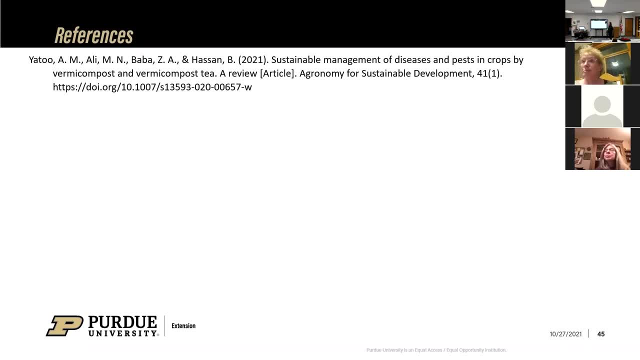 Now good thing is happening. If you notice, they're starting to do more with the cover crop Now. I'm seeing more of that right now, since the beans are being harvested. We started looking at the bean fields around right now. You're going to see a lot of green coming up. 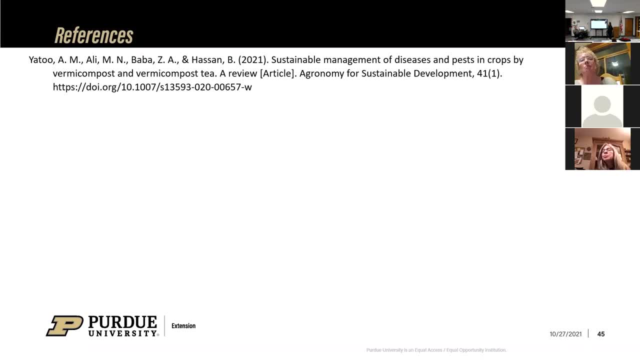 because they're all going in there and starting to put a cover crop on That kind of spring. they'll put a burndown on there and then they'll plant. no-till They'll plant corn, So also that gray stuff might also be. 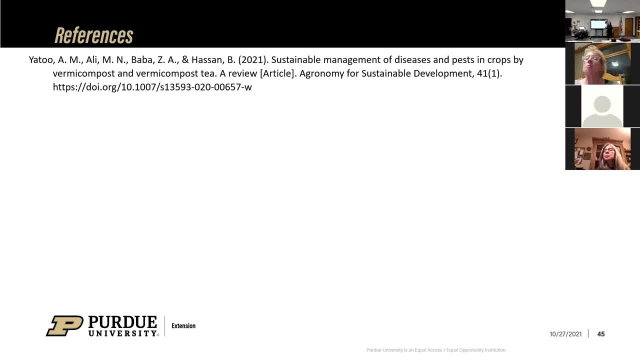 gypsum Gypsum is not lime Gypsum. yes, that is different. It does look similar, but it does not raise the pH. It's more about soil tilt, It's about the soil texture. That might be part of it. 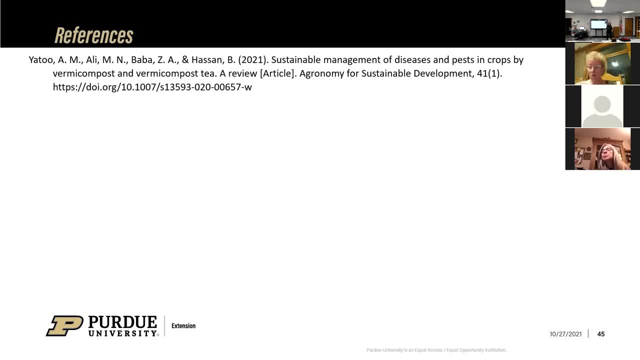 Plus, farmers right now are dealing with a lot of water so they don't want to have compaction. That might be part of trying to probably prevent that compaction in the spring. That big equipment now really does compact the soil a lot. 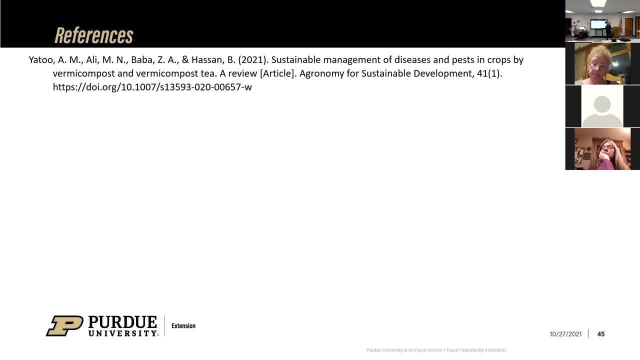 They're just trying to get the fields clear. The rain is going to keep them out of the fields, Whatever it takes. they may have to have ruts and they may have to get the compaction, but they're just trying to get the corn fields out. 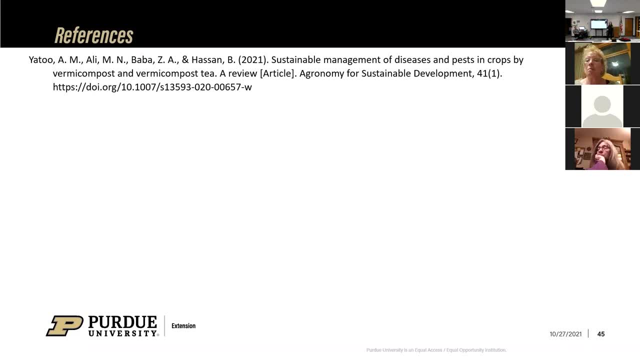 Doesn't the gypsum break up the place for it? Uh-huh, Yeah, it basically makes that tilt. That might be what's happening, I'm not sure. Yes, Greg, I have a question for the poop lady. Yeah, poop lady, That's right. 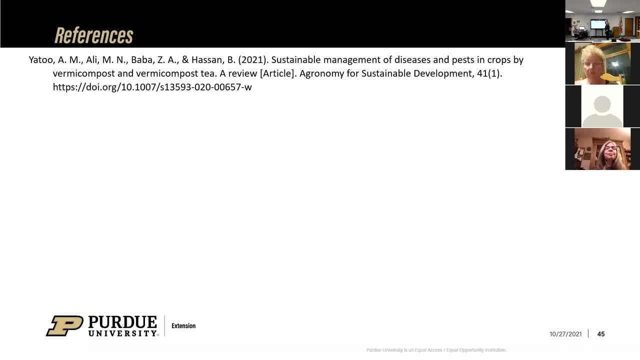 In your backyard little compost pile and your little house pet that poops on it. what is it? What's your position on if you put any of that in there? Okay, If you're going to compost your dog, you wouldn't want to use that on your vegetable garden. 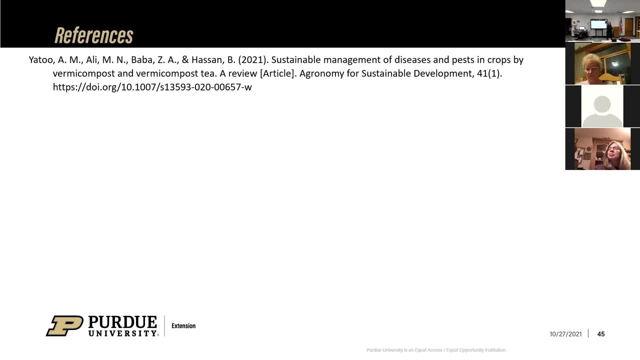 Because, depending on that disease that your dog could have- I'm not saying your dog is diseased, but let's say it is- we can get the same disease, especially the same worms. You can totally put that on your ornamentals. Okay, Anything other than a vegetable garden. 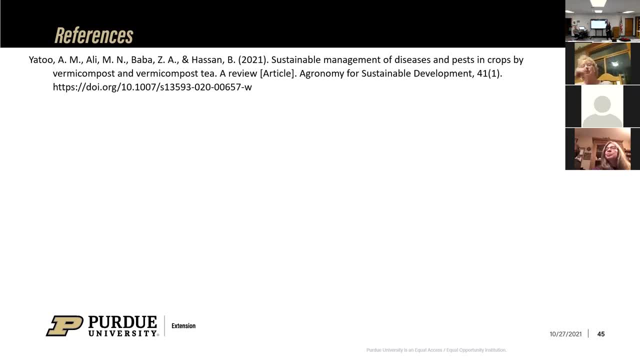 Correct. Yeah, it's got the eco. Yeah, it's got the eco and other fun worms, Because I'm guessing you give your dog a hard-worn medicine every now and then. No, I don't have a dog, Okay, Well, you give your dog a hard-worn medicine regularly. 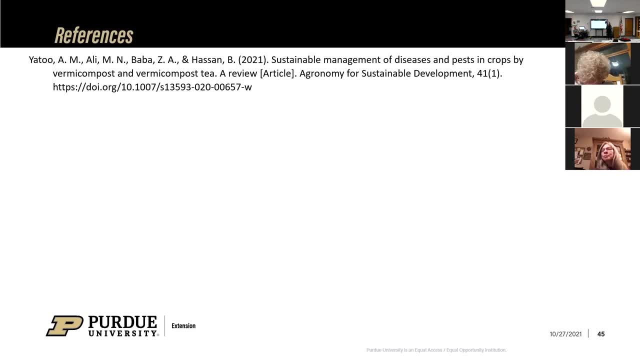 because here's the deal: they're always going to have worms. They always have worms and you don't want them. I don't know. You just have worms, I'm just kidding. I have them, Yeah, but not dog worms. 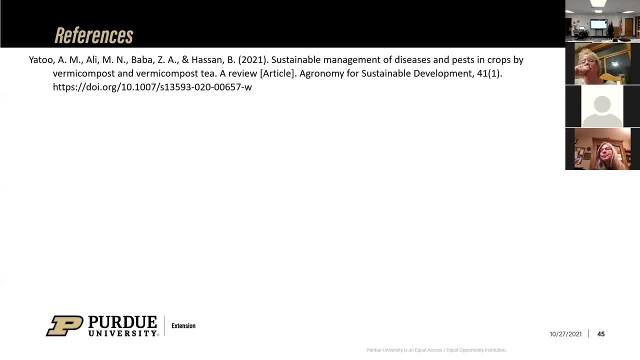 People have worms. I know It was kindergarten. They're so gross, But the dog can walk through it. That's a good point. They might have other questions. Yeah, but wasps can pollinate, but they're also predators. 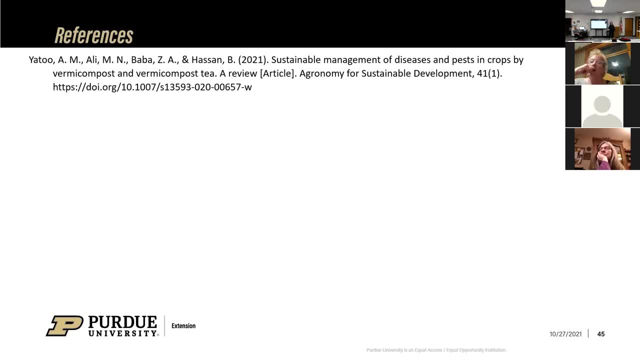 and they're eating like they're bad caterpillars. They are taking your caterpillars and feeding their babies. They're carnivores, but they also do eat nectar for energy, just like we like carbohydrates and proteins. They're the same way Wasps do play a good role in the ecosystem. 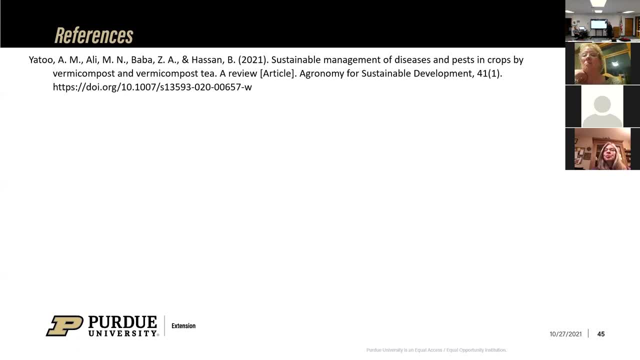 but don't step into their nest. They're going to watch where you're going. Yeah, They're going to watch people. Wood bees or pollinators. Wood bees or pollinators? Yeah, Dawn, how do flies are pollinators. 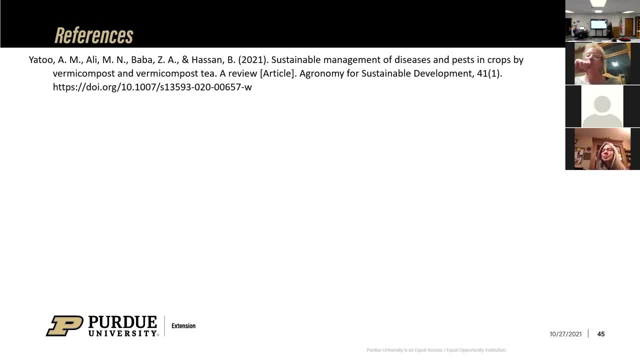 You know what they're doing to it, don't you? Yeah, Yeah, I can see that. Yeah, you have to sometimes do what you have to do. Yeah, Carpenter bees, Carpenter bees. Yeah, I know everyone hates carpenter bees. 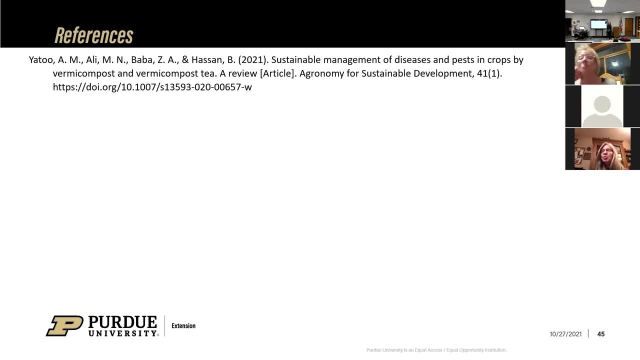 Yeah, Bald-faced hornets, Bald-faced hornets. Yeah, I saw your hornet nest, but they do freeze out. Yeah, with the frost. But you know people buy those nests. Yeah, They'll buy them. Anybody have any other questions at home? 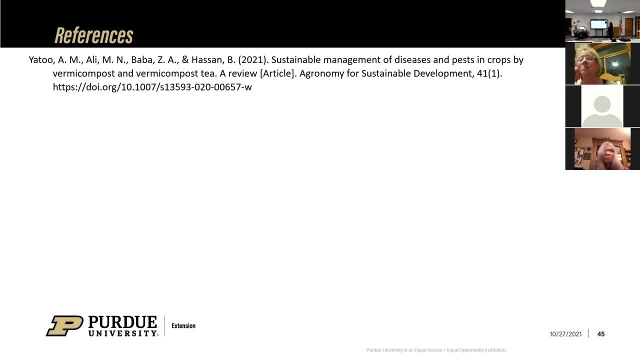 I can hear you at home if you want. Hope you can hear me. She's going to the back. That's it, Vicki, She's going to the home. Thanks so much, Ray. Really good, A lot of great information. 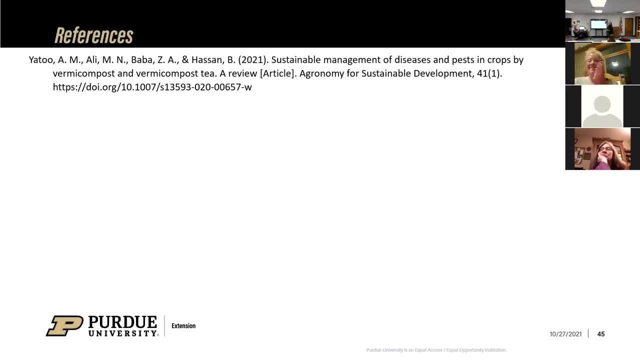 Thanks guys for being here and it'll be recorded, but if you have any questions, just let us know. Thanks guys for being here and it'll be recorded, but if you have any questions, just let us know. 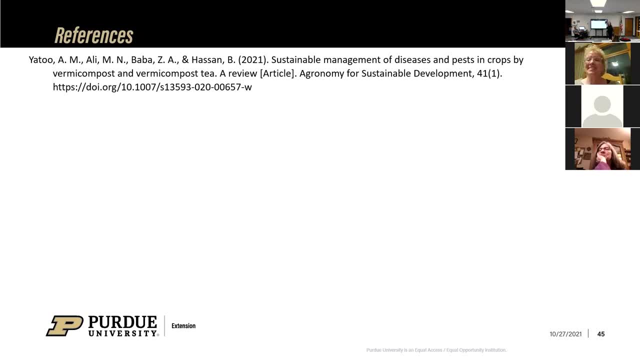 Thanks, guys, for being here, and if you have any questions, just let us know. It'll take me a few days to do that, you know, and Teresa will send it out. So thanks so much for being here, Great. 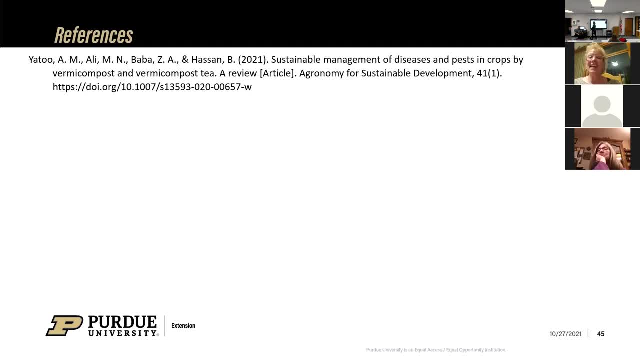 Thank you. Thanks for being here, Take care. Thank you, Go around and do it So I know where I was going to answer And you'll know where I was going to answer. Okay, Got any rules? We'll go around and ask for them.